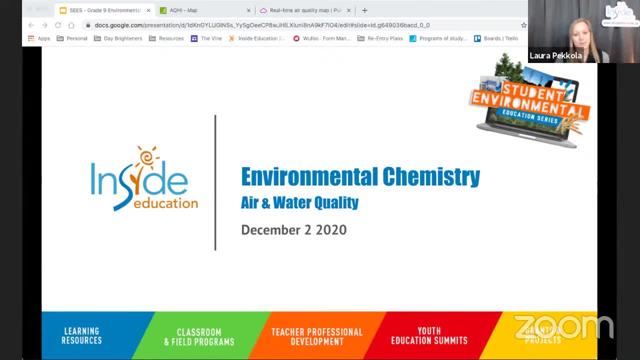 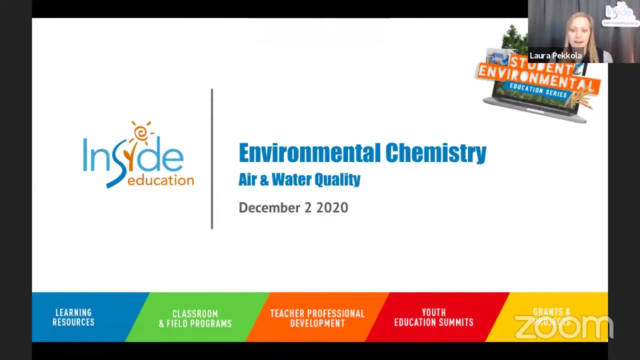 topic of the topics of environmental chemistry and especially air and water quality, and take that forward into an idea of environmental stewardship. So I am, as I said, in Edmonton, which is traditionally known as the Miskwitchie-Waskehegan on Treaty 6 territory, which is the traditional lands of the Cree, Soto, Blackfoot, Dene and the Kota Sioux peoples, and this is also part of the 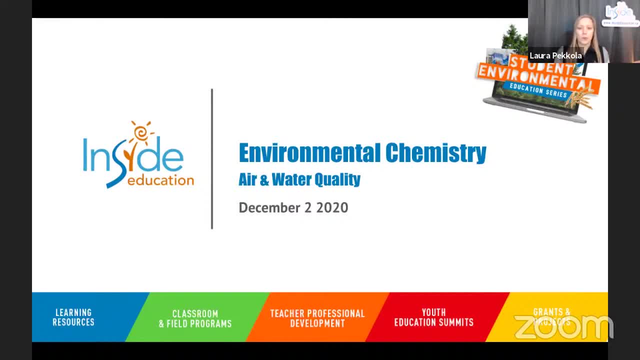 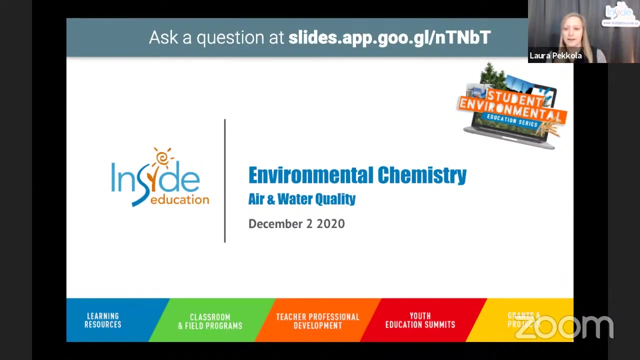 Métis Region 4, as well. So we are here again on our last Student Environmental Series presentation, which is really, really exciting. I have just a couple things to get us started. so you'll notice that there is a there is a question and answer URL. that is on the slide. You can find that there too. 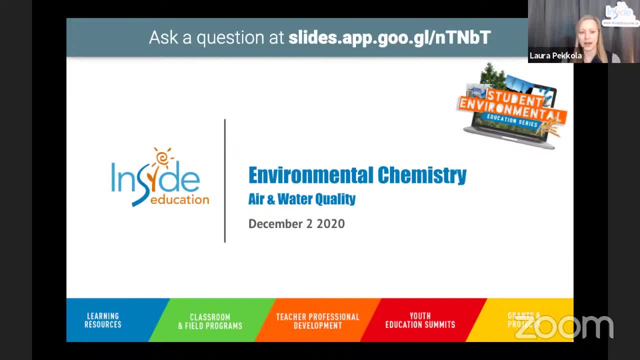 can see, and also, if you're joining on YouTube live, you can actually access that from the link in the description. So this will be the best place for you to post any questions that you have as we go through this webinar, and I will be checking it periodically If you are joining on Zoom. 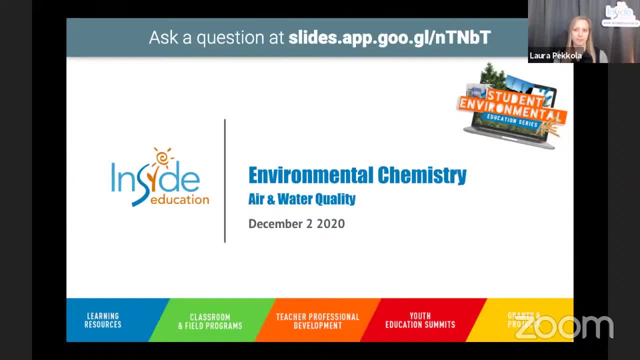 you can use the chat in Zoom as well. So today we are going to be talking about air and water quality. but why? Why do we even care about air and water quality in the first place? So I know for myself. I love to play outside, so I think it's really important for us to know. 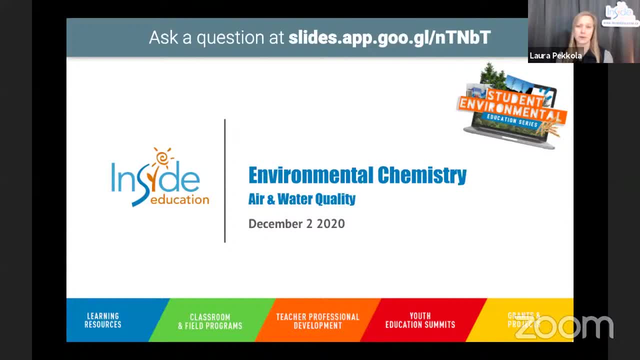 how healthy our air is and how healthy our water is, especially if we're spending a lot of time in it. The reason for that is that both air and water can affect our our health, so we need to know how that effect can happen. And I'll throw this one in too: I think nature is absolutely beautiful. 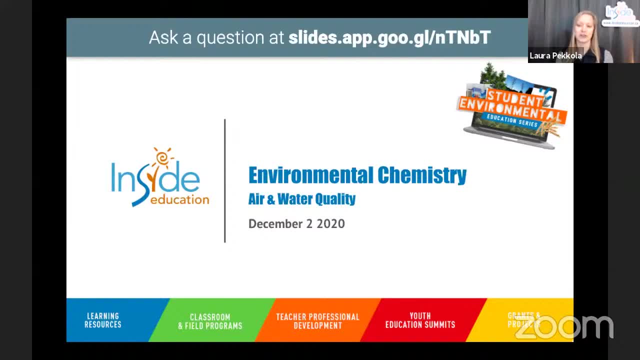 and we have an inherent responsibility to make sure it remains healthy, not only for ourselves and for other humans, but also for the plants and animals that make it their home. So we're going to explore responsibility, being stewards or caretakers of our water and our air, and I think the first way. 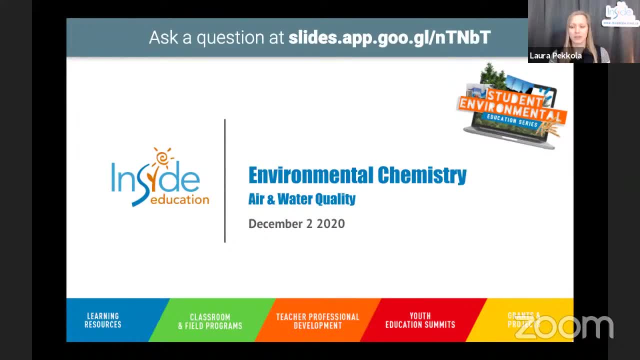 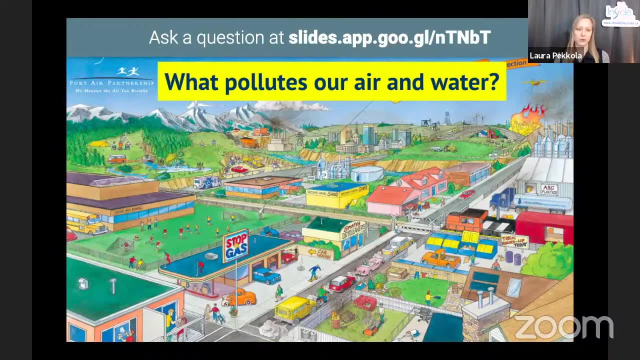 that we can ensure that we are, that we are doing this is just seeing where those pollutants are even coming from and what those pollutants are. So I'm going to put up this slide here and put it out to all of you who are watching What actually pollutes our air and water. So, looking at this, 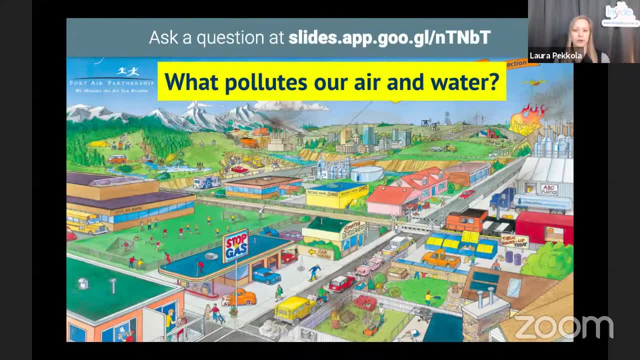 image. what are some of the sources of air and water pollution that you can see. If you want, feel free to put them in that Google Slides Q&A and and I can take some of the questions that you may have, So I will just go through some answers there. Also, I want to mention that this is a pretty 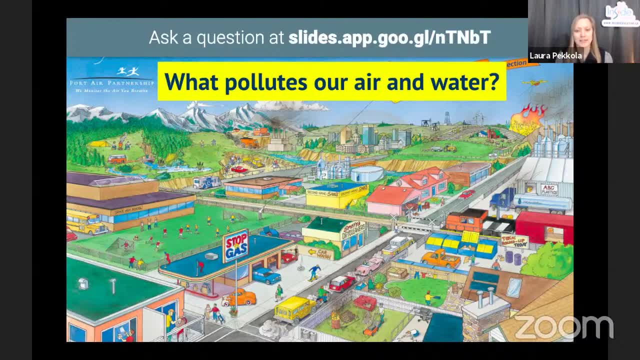 typical landscape in Alberta, So in the background you can see that there's a pretty big city, something like maybe Edmonton or Calgary. There's farming, forestry and oil and gas extraction taking place outside of the city, as well as some components of a sample neighborhood in. 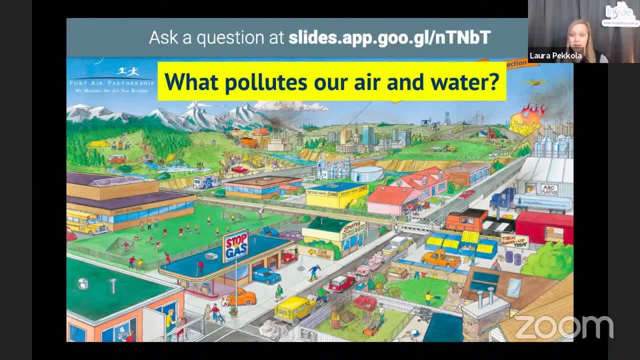 the foreground, which probably look pretty familiar to you: So many ways in which our everyday life can add sources of pollution to the air and water, and I'll just see if anyone has come up with any. Don't see any yet, So I can start my big reveal and start going through some of the ones that I 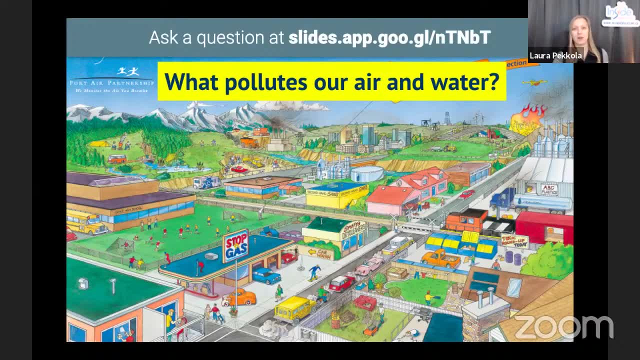 have thought of. So as we go through these, you might hear of some compounds, some chemicals that you haven't heard of before. That's totally okay. I just think it's really important for us to know exactly what it is that's in our environment, for us to understand it better. Oh, I'm seeing cars. 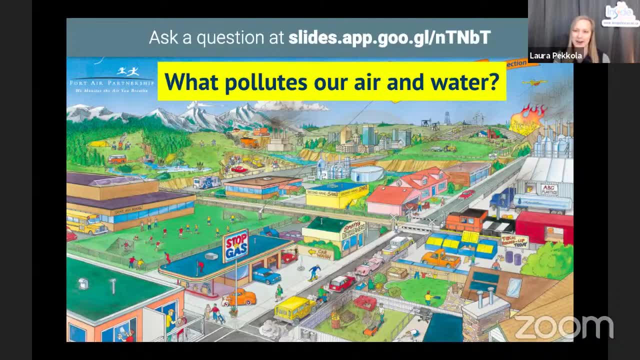 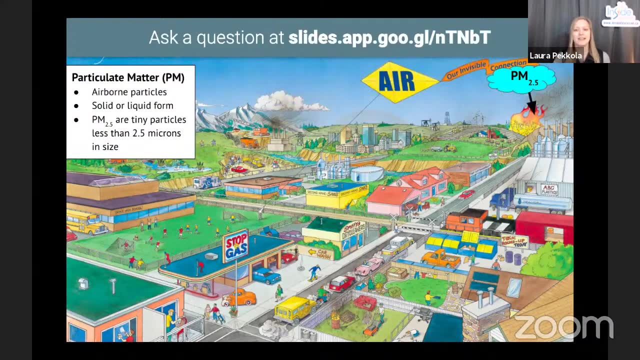 forest fires. those are awesome Examples, thank you. thank you for those who are putting those in. So forest fires is actually the first one I wanted to point out. So up in the top right corner you'll see that there's a forest fire. 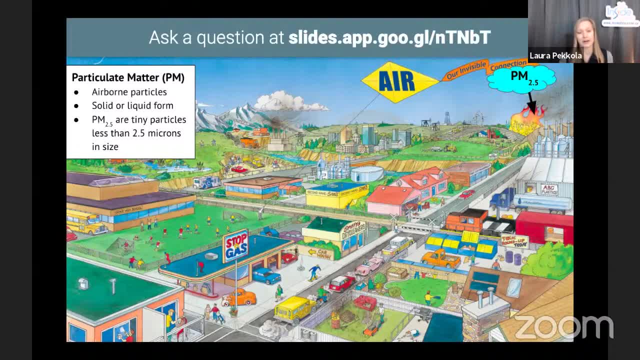 and one of the main things that forest fires contribute is particulate matter. So particulate matter are really really tiny pieces of either solids or liquids that are airborne. So usually they are formed as a result of a chemical or physical reaction and in this case, and you know, 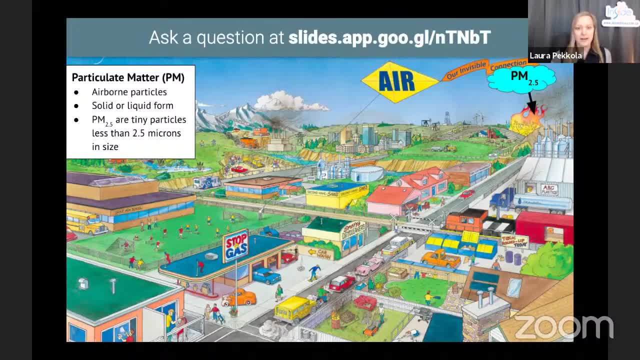 often it is because of combustion or burning. So you'll see that there's a little 2.5 next to the particulate matter. So that just means that that particulate matter is 2.5 microns in size or smaller. So that is really tiny and really hard to actually to actually understand how big it is. 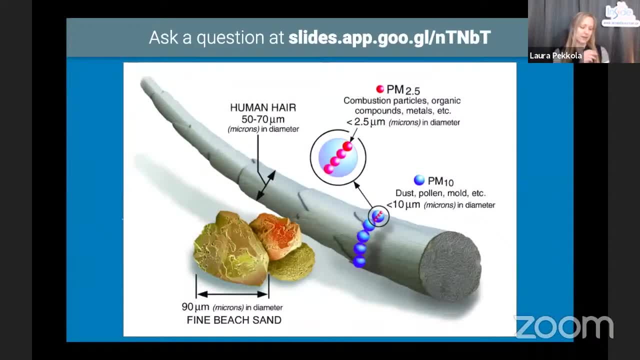 So let's take a look at this. So, if you look at the width of your hair- pretty small in itself- well, pm 2.5 particles are 1: 20th the width of a typical human hair, So they are quite tiny. They're the red balls. 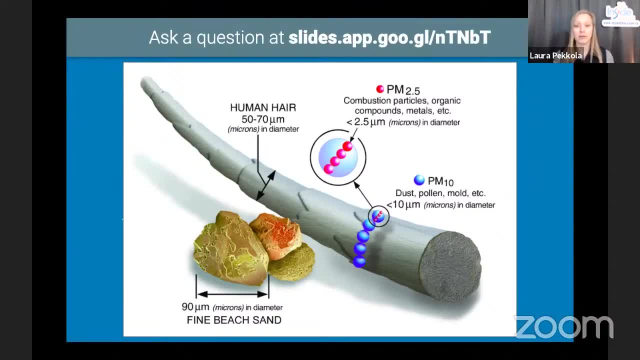 that you can see on that on the photo there, okay, And then pm 10 are also particles that we can inhale, but so they can still enter our lungs, but they are a little bit larger, So they're about the fifth of the size of a hair. The problem with particulate matter is that it can get all the way. 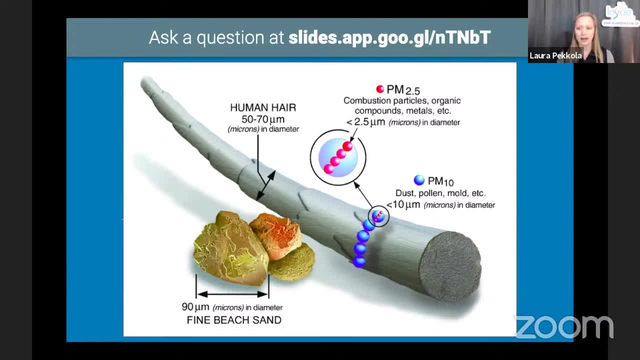 into the alveoli or the hair follicles, So it can get all the way into the alveoli or the hair follicles Or the air sacs in our lungs, which is where the oxygen goes from the air that we inhale. 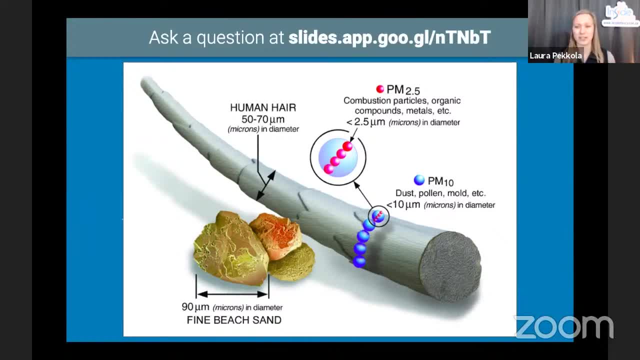 into our blood. So if we get a lot of this teeny tiny particulate matter into our alveoli and into our lungs, it can kind of clog it up and it can mean that we can't quite get enough oxygen from the air into our blood. So that's one of the reasons why we care about. 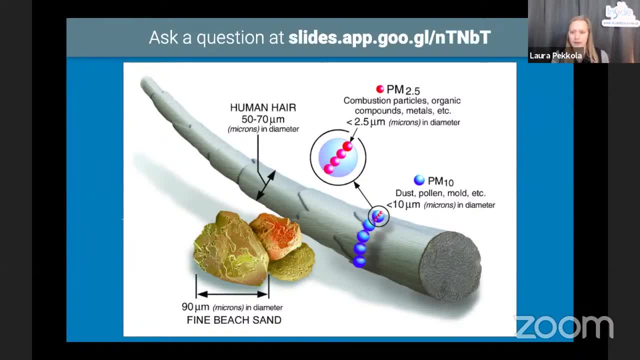 the particles that are in the air. All right, let's see our next one. So the next one we're going to look at is the alveolus. So the next one we're going to look at is the alveolus. So the next one we're going to look at is the alveolus. 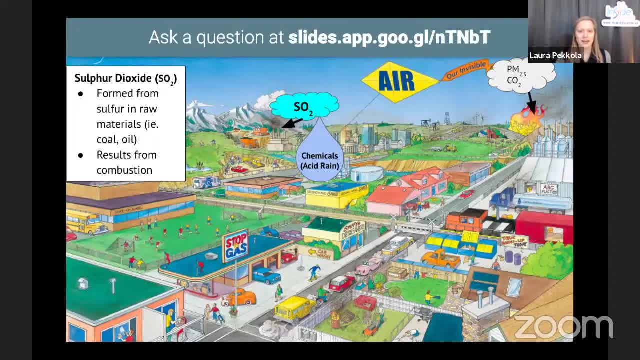 at is sulfur dioxide. So sulfur dioxide is formed from sulfur in raw materials, especially when we burn it. So those raw materials are generally our fossil fuels, because fossil fuels are naturally quite high in sulfur. So when it goes into the air it can combine with water vapor and it can 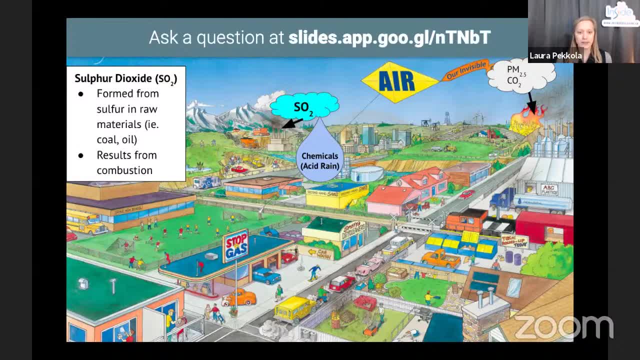 actually cause acid rain. That's why you'll notice that on the screen there there's a little water droplet that has the chemicals- acid rain- written in it. So as we go through these examples, the chemicals that are put into the clouds, those are air pollutants. And then, if I add a water, 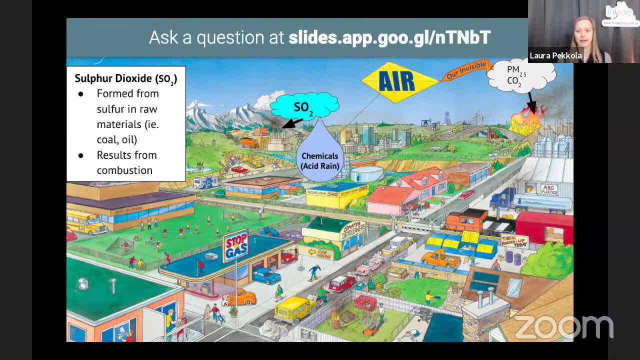 droplet on it as well. that means that water can be polluted by that as well, So sulfur dioxide can come back down into our water system through that acid rain, which is a bit of a problem. We're going to talk about how industries have made. 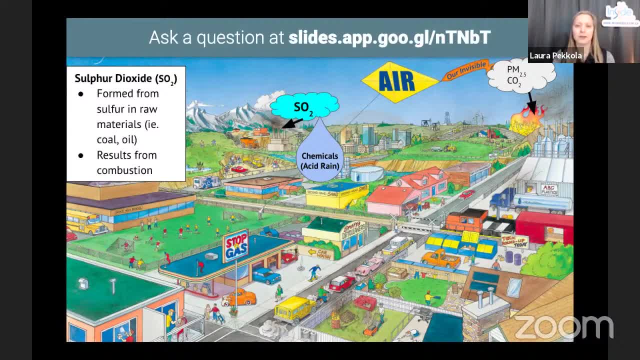 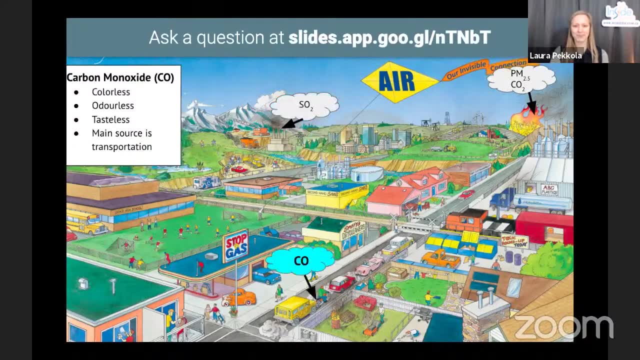 maybe started fixing some of these problems a little bit later. So don't worry, even though that is a cause, it's not a hopeless situation, Don't worry. So next we have carbon monoxide, So this can come from the cars that were mentioned as one. 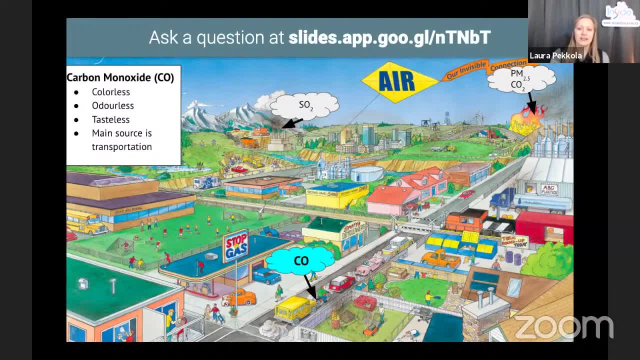 of the sources earlier by one of you. So when we have incomplete combustion in gasoline engines, we can get carbon monoxide coming out into the air. And carbon monoxide is colorless, tasteless and odorless. So it can be really dangerous because you don't even necessarily. 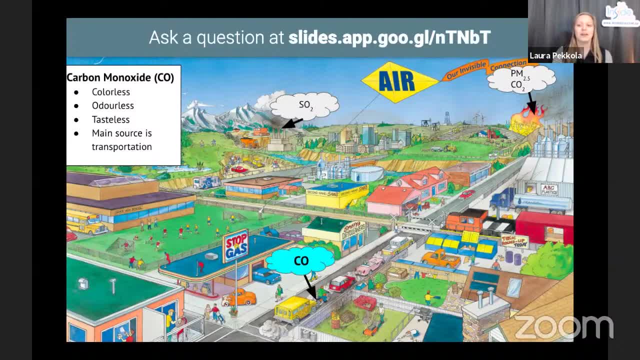 know that you have a lot of it around. So that's why we have carbon monoxide monitors inside of our homes, because we need to make sure that we are monitoring for it in our homes so that it doesn't make us sick, But it can also be a problem out in the environment as well. 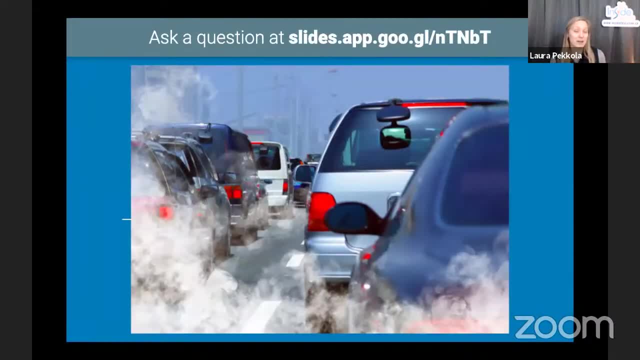 So car exhaust. regardless of whether you can see the exhaust coming out of a car or not, if it is a gasoline engine, there is some carbon monoxide coming out of there. as well as this other, this next pollutant there at the bottom called nitrogen dioxide. 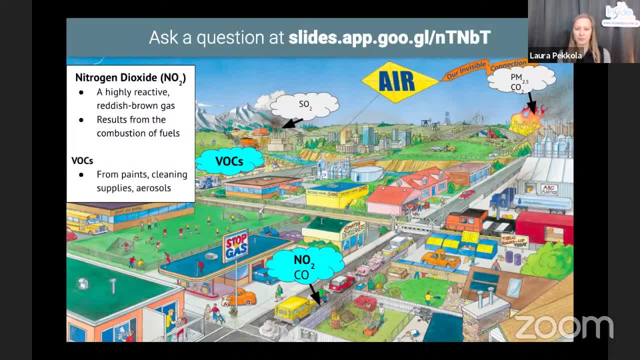 So nitrogen dioxide is highly reactive. It's a reddish brown gas, though we don't usually see it in high enough concentrations to see the red and brown, And it results from the combustion of fuels as well. You'll notice I put up another chemical there. 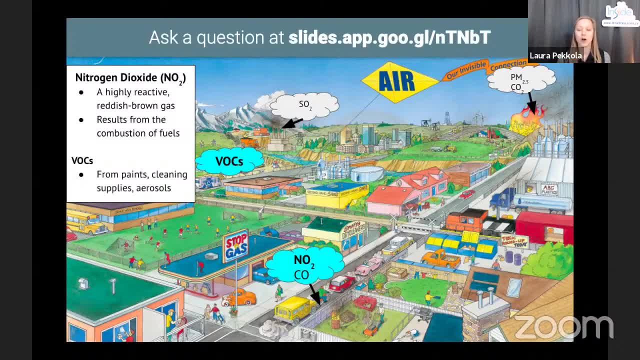 at the top, called VOCs. So VOCs are volatile organic compounds and they actually come from things like paints, heat cleaning supplies and aerosols. They can also come from natural sources such as plants. So volatile organic compounds, along with many of these other compounds that 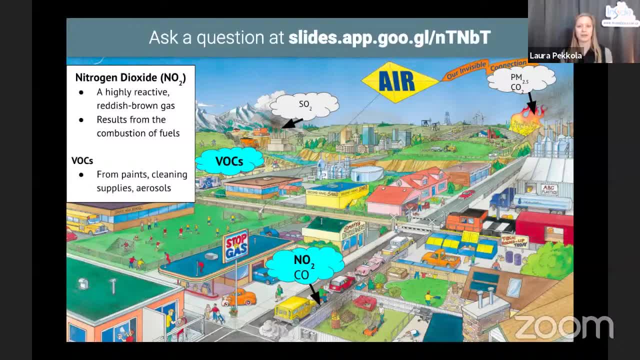 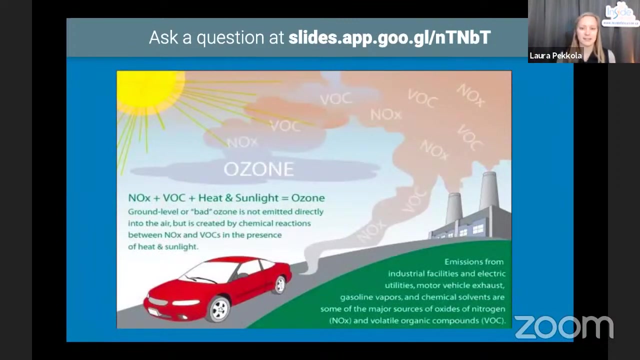 we're talking about. they exist naturally in our environment. It's just the fact that human activities can increase their concentrations in the environment to something that's not healthy for either humans or for the environment either. So the interesting thing about those VOCs and nitrous oxides- 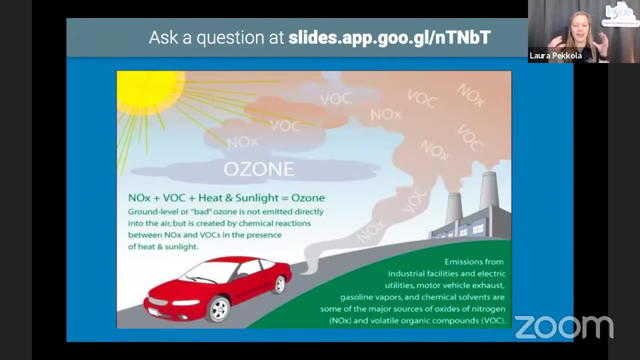 so the NOx that you see on the photo now is that they can actually go through a chemical reaction with each other when there's enough heat and sunlight to produce ozone. So when the emissions are right, these two pollutants can come together to make ozone. You may be. 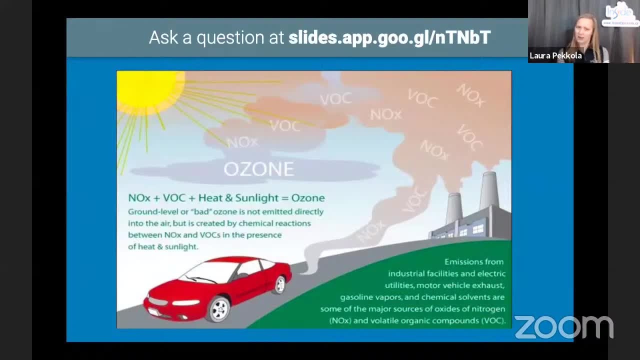 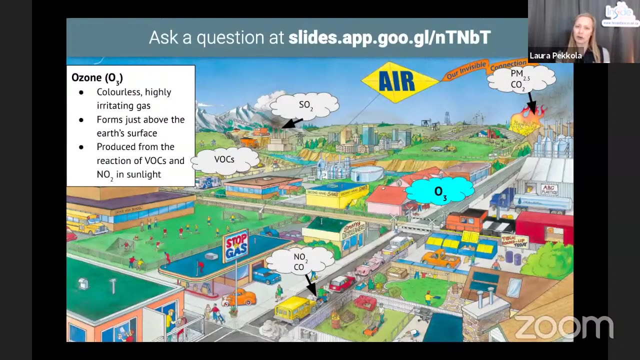 thinking: hurray, I've heard about holes in our ozone layer. This is an awesome thing, right? Unfortunately, not because this form of ozone can be dangerous just because of where it is. So ozone is colourless and it's highly irritating to our breathing and to our eyes. 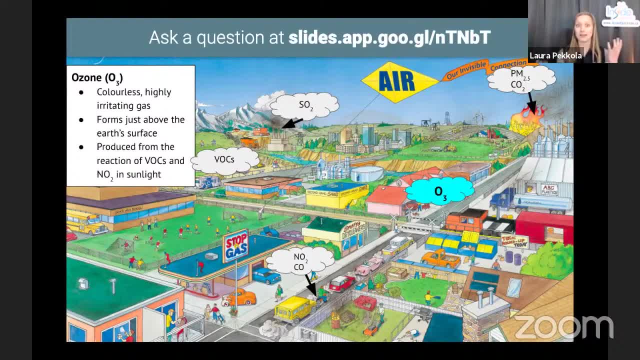 And when it's at ground level as it is, when those nitrous oxides and volatile organic compounds combine, it's right here where we're breathing. So that's the problem. It's still the exact same compound as up in the atmosphere that is keeping those UV rays or kind of filtering out. 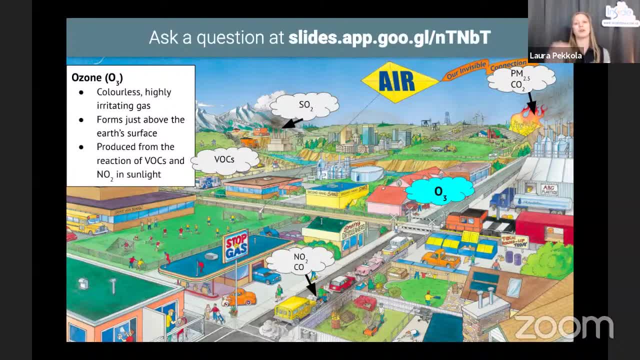 those UV rays, which is good for humans, but when it's at ground level not super great for our breathing. So therefore it's considered a pollutant. The interesting thing about ozone because it's produced in this, in this reaction between nitrous oxides and and volatile organic compounds. 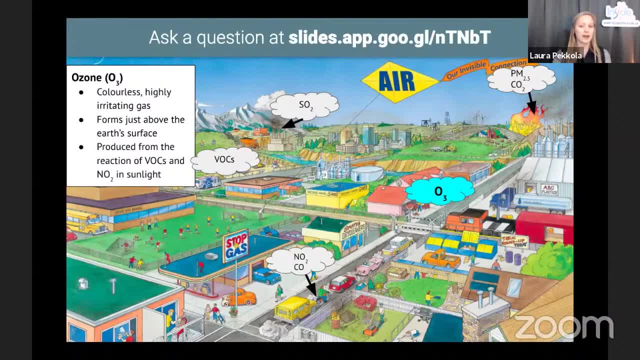 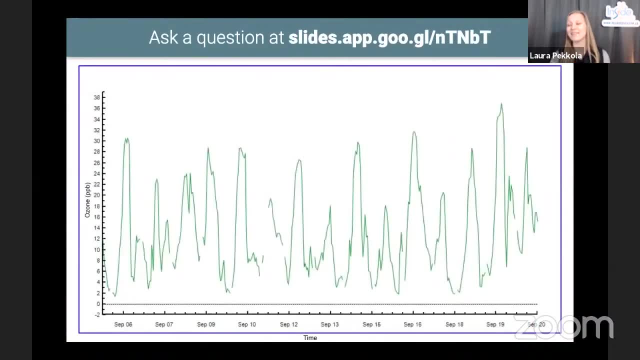 is that we often find it in places where there's high traffic. So I want to show you this graph and I want to challenge you to try and interpret this graph before I give you the answer. So here is a graph of ozone concentration over a two week period. This measurement was taken in Fort. 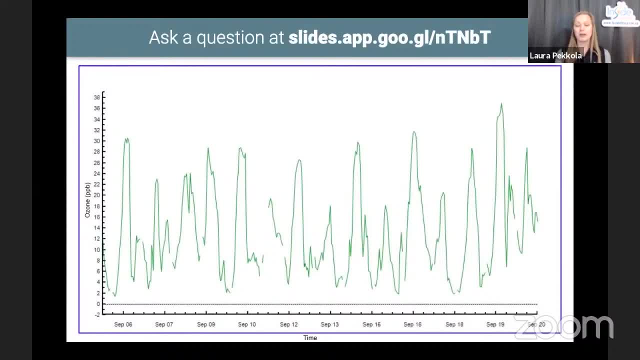 McLeod Murray, very close to the center of town. So so right where people are living And you'll see that there is a little bit of a pattern here. So I know the time is a little bit tricky to to keep track. 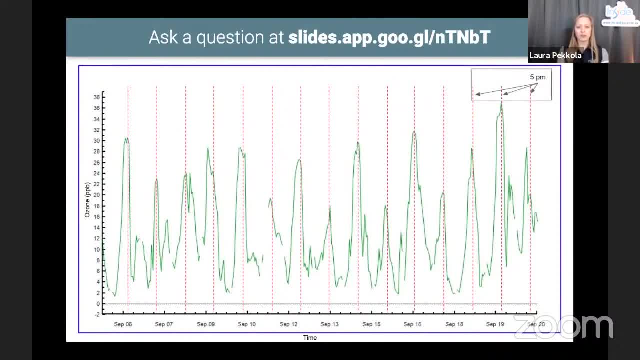 of So here I'll add some lines here. So each of those red lines corresponds with 5pm on each of the days. What do you notice about that ozone pattern? You might notice that the ozone pattern tends to peak at that 5pm time. Why would that be? Well, the thing is, around 5pm people tend to be. 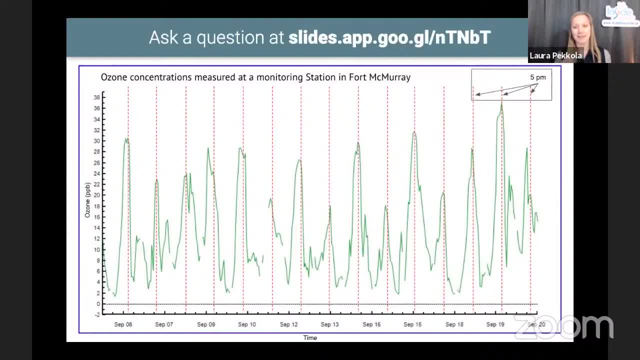 driving home from work. So it makes sense that if there's higher traffic on the roads then that ozone is also going to increase because there's all that nitrous oxide coming out of the car tail pipes and and then is being formed into ozone. My guess during these two weeks is that the weather 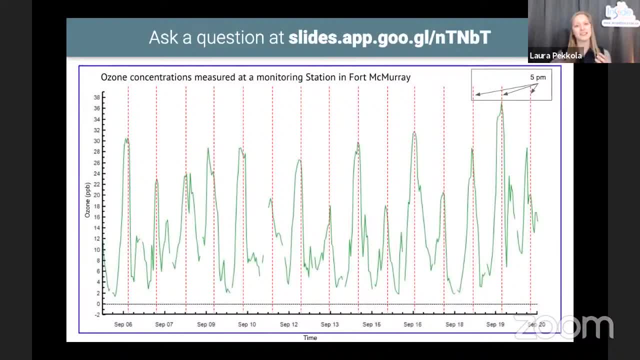 was probably quite sunny And so, and then it's going to be higher traffic on the roads, And so we're going to have to wait a little bit longer to see if it's going to be as sunny and warm, because that's the conditions that allow for nitrous oxides to really be produced in in the 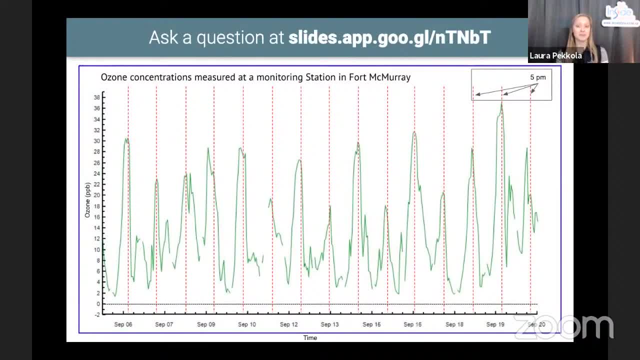 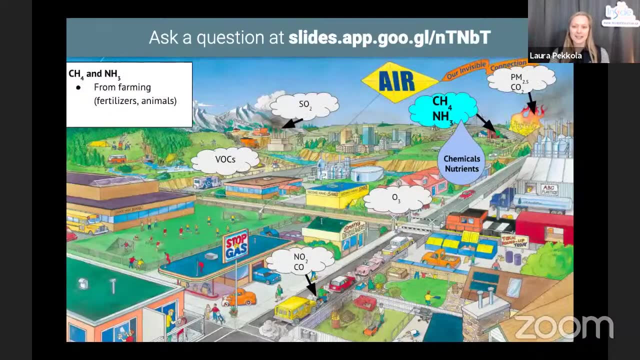 most efficient way, I guess. So if we went back to September 2019, my guess would be that the weather during that time was quite warm and sunny. One of you can can do a fact check on that for me to see if my hypothesis is correct. All right, a couple more to look at. So farming can also. 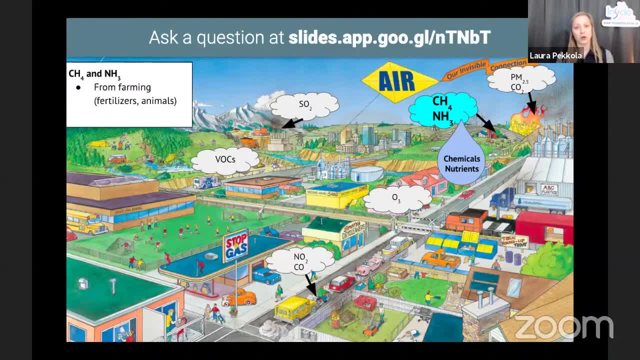 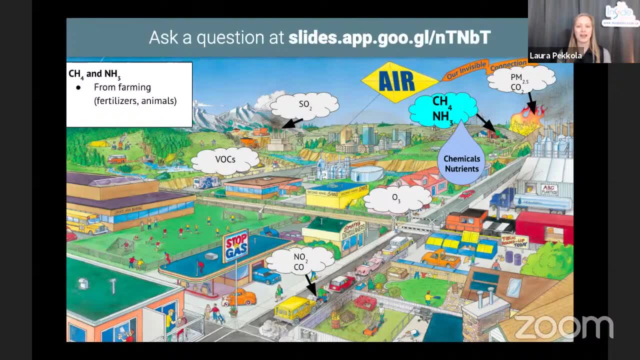 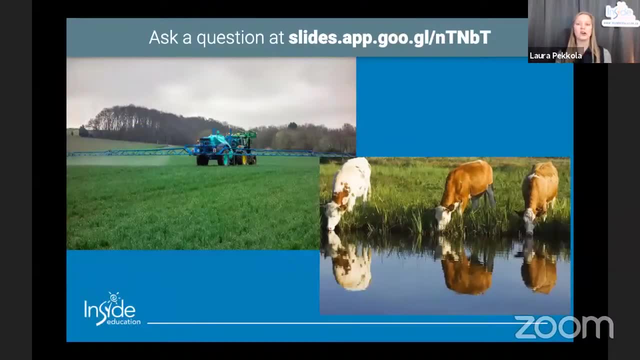 ammonium which can be added, And they can come from the fertilizers as well as from cow digestion. So when cows digest their food, they burp and fart out methane, which can then end up in our environment. In terms of the ammonium from fertilizers, it can end up out in the air. 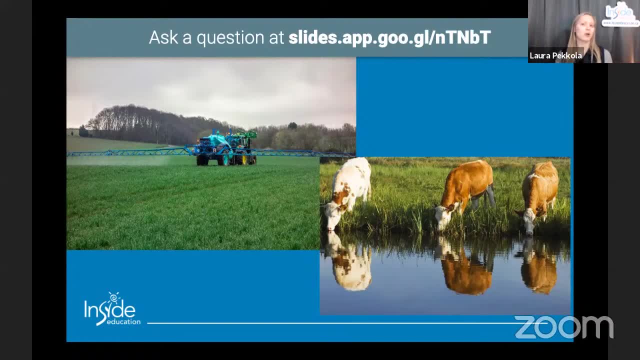 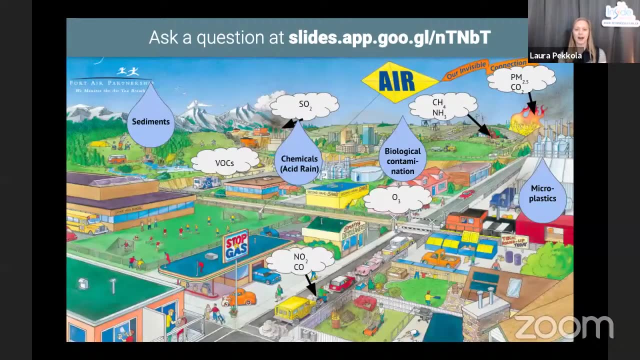 but then it can also end up in the water and then going down into groundwater or running off into surface water areas as well. So here you see, the majority of the pollutants that we're going to be considering today and what those sources- sources of pollution- were. So if you 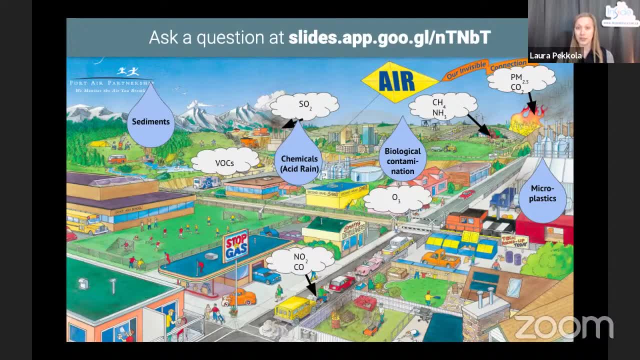 have any questions about this or anything else as we go through this presentation, remember, don't hesitate to use that Q&A link that shared at the top of the presentation, and I'll do my best to answer those. Okay, so now that we know a little bit about what is causing the pollution in our environment. 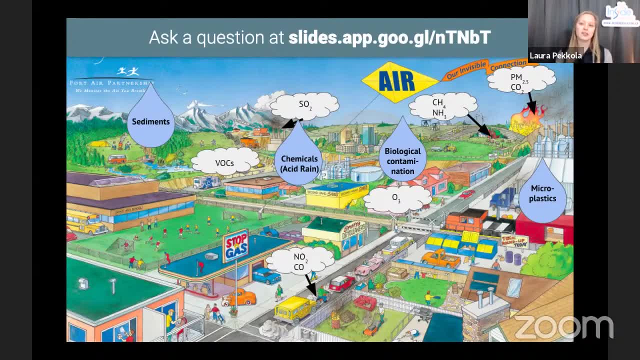 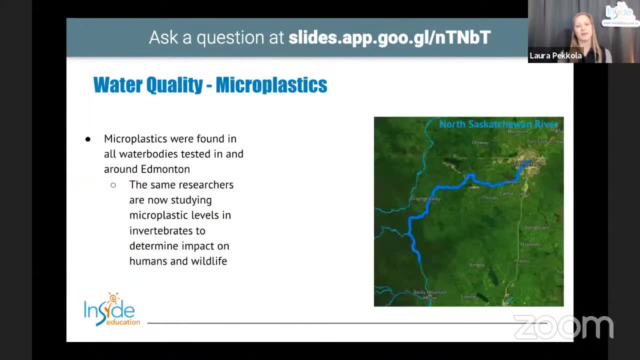 I want to look at some case studies right here from Alberta to delve a little bit deeper. So this first one actually has to do with microplastics, which we didn't really talk about, but maybe you've heard about in in your everyday life. even microplastics are in the news. 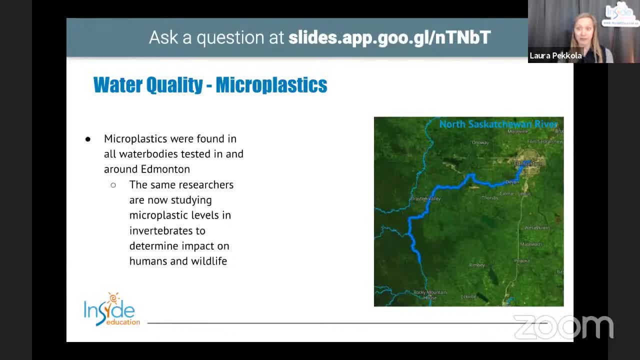 quite a lot because they are very, very prevalent. So this was a study done by MacEwan University and they found that there were microplastics in all water bodies tested in and around Edmonton. Why do you think there would be so much microplastic in the water bodies in and 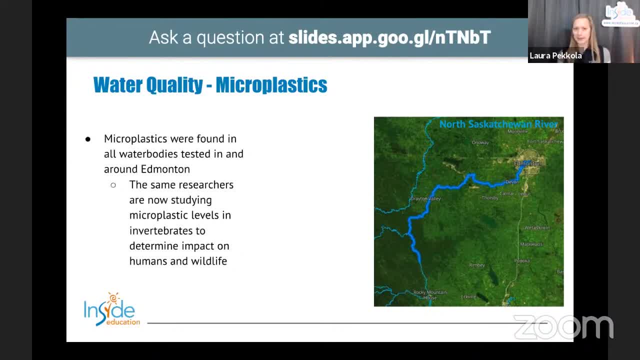 around a basin city like Edmonton. Where would those microplastics be coming from? Well, microplastics can come from any source of plastic. really, When we recycle plastic, we think that it magically disappears or it all is formed into a new form of plastic and it's great for the environment, right? 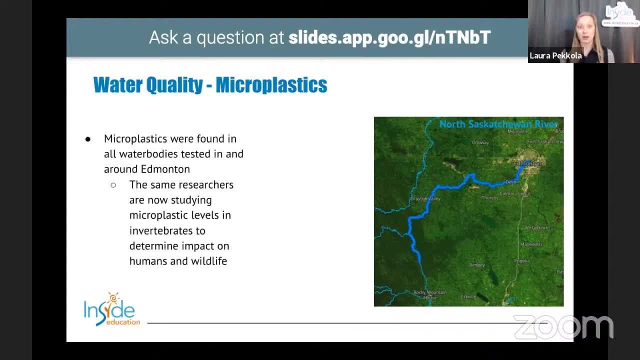 But plastics they shred really, really tiny particles off of them all the time and those end up maybe being washed down the drain, even maybe just out on the road, if you think about tires and the plastic of a tire kind of wearing away slowly, and they do end up in our water bodies. So 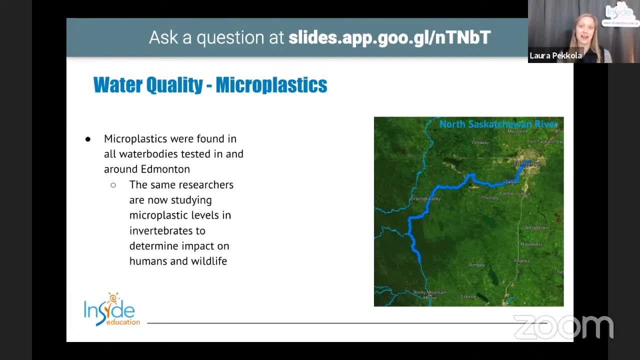 even our clothing can cause microplastics to end up in the water, because every time we wash our clothes, if you have something like a polyester or any other synthetic material, it can shed off tiny bits of plastic which then end up in our water. So the next step that 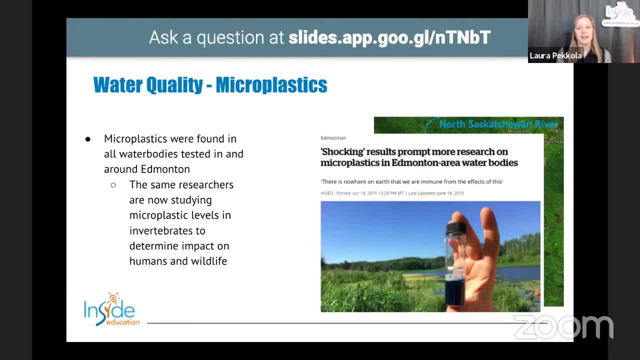 that these researchers want to take is to look at the levels of microplastics in some of our invertebrates, and the reason they might want to do that is that invertebrates are those teeny, tiny pond critters that you might have caught when you were doing wetland. 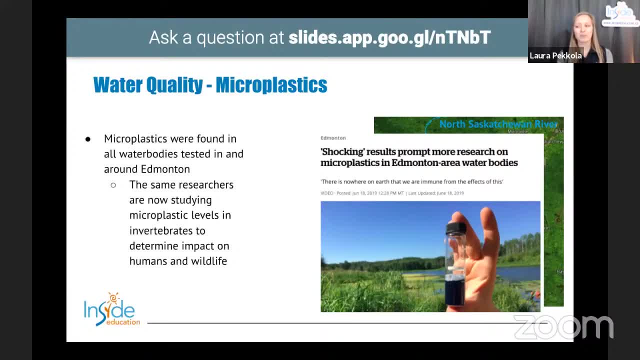 studies in the past. but they are kind of at the bottom of the food chain, if you think about it. So if these little micro, or if these invertebrates have microplastics within them, What happens when, say, a fish eats a whole bunch of these invertebrates? 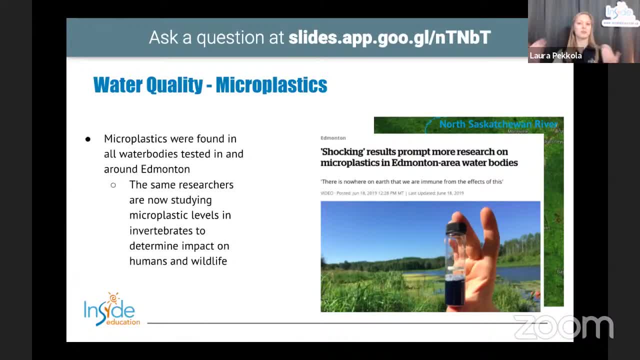 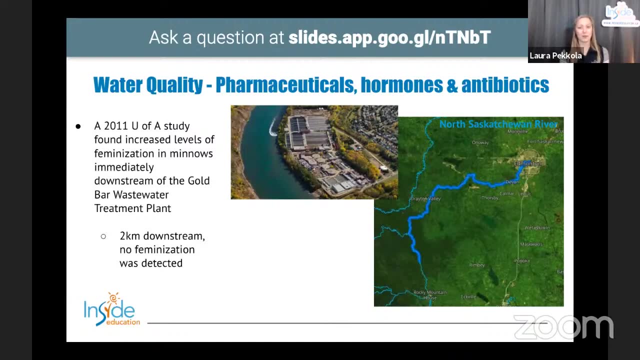 It will also end up with those microplastics inside of it, So it can actually result in maybe a lot of high concentration being concentrated in these animals higher up on the food chain. Now, another thing with water quality is that we can actually end up with pharmaceuticals. 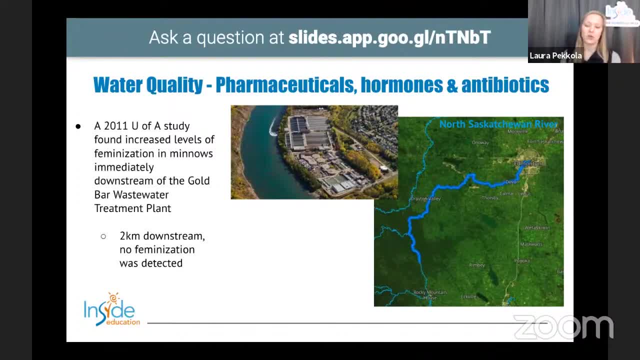 hormones and antibiotics in our water. So in 2011, a? U of A study found increased levels of feminization, which means that the proportion of females to males in the population was much higher on the female side than on the male side, and directly downstream from the Gold Bar wastewater. 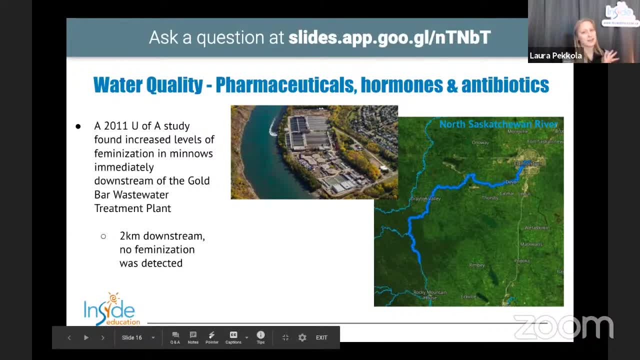 treatment plant. Then when they studied it two kilometers further downstream, they didn't find that effect anymore. Why would that be So? you may have heard the solution to pollution is dilution phrase before. I don't think that's the solution to pollution at all, but it is something that happens Once you get a pollutant. 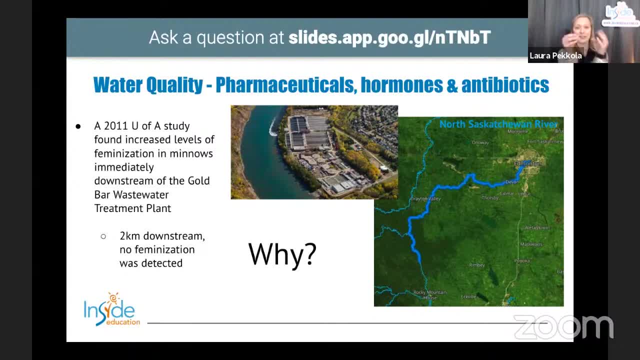 out into the environment. it means that it doesn't just stay right where it's emitted, It spreads out. It spreads out in the air, it spreads out in the water and eventually it gets to a low enough concentration that it doesn't have the severe effects that it has when it's really really localized, or right. 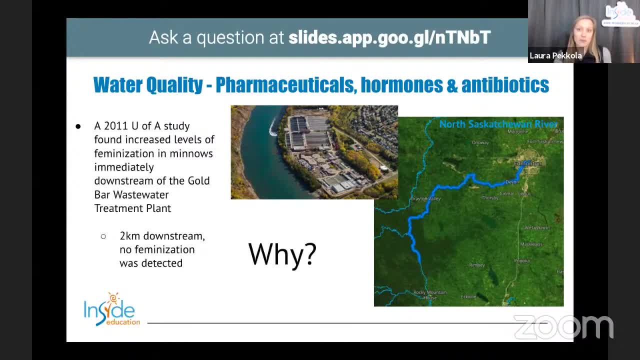 where it's emitted. So with this, the thing with these hormones and medicines that go through our bodies is that they actually often end up going through our body, being flushed down the toilet, and then they aren't always cleaned up by wastewater treatment plants fully, so they can. 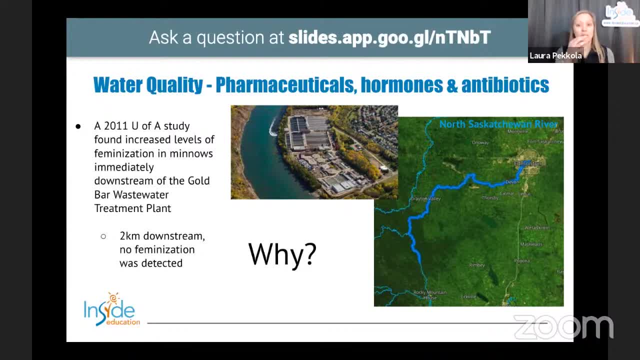 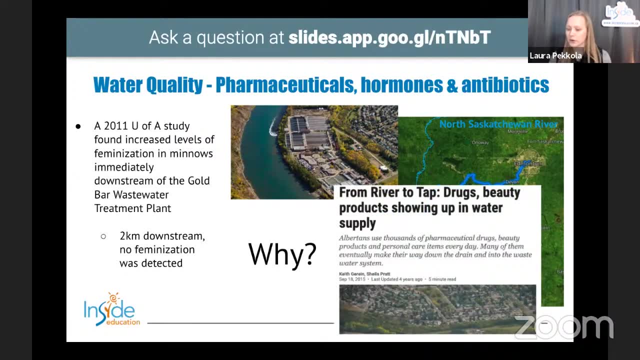 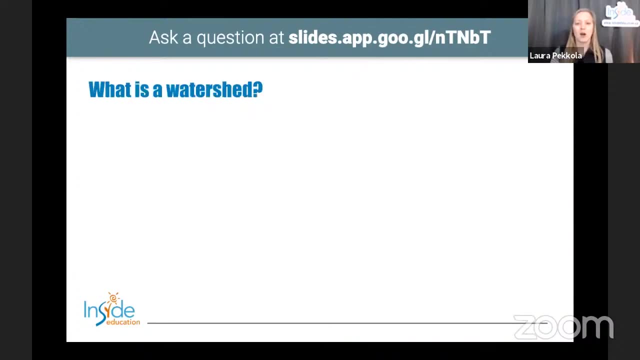 end up in our rivers as well. So those medicines and hormones are ending up in our river bodies, but they tend to be diluted once you get far away from the wastewater treatment plant. Does that mean that we don't need to worry about that? Well, not necessarily, because we're all connected in our watersheds. 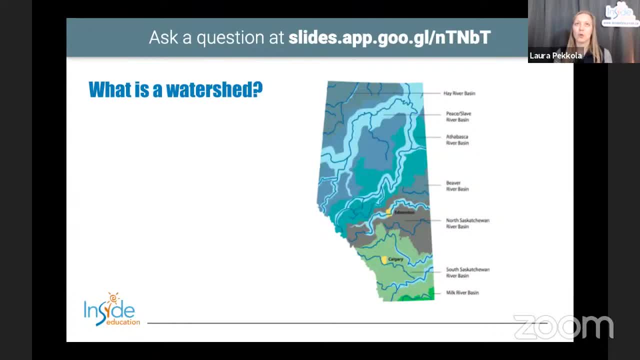 So if you tuned in a couple weeks ago to the water presentation, you would have heard a lot about watersheds and some of the water quality challenges that are associated with water in Alberta. So I'm not going to go into too much detail about that so you can go back to that presentation on our YouTube channel if you're interested. but I do want to go through some of these: this concept of a watershed and what that actually means for what we're putting into the water. 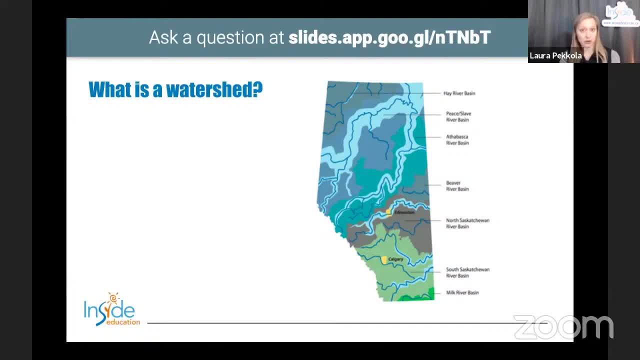 So in Alberta we have seven watersheds. so assuming you're joining us from Alberta, you're going to be in one of these seven here and they all drain to different, or they drain to various areas of the ocean as well. So at the top, 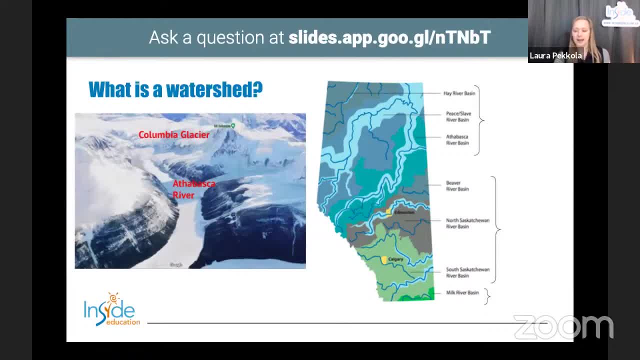 you see our Hay River, Peace and Slave and Acabasca River basins. They are fed by the Columbia Glacier. So the Columbia Glacier is the headwaters and then all that water, or from that glacier the water travels west through Alberta and it actually continues north. 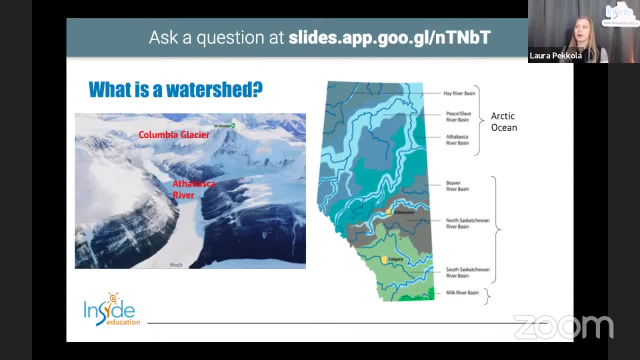 up to the Arctic Ocean. So let's think about a city that is within that area. So, for example, Fort McMurray. I used to live in Fort McMurray. I know that Fort McMurray is in the Acabasca River Basin. So anything that happens in Fort McMurray, or any other chemicals or anything, 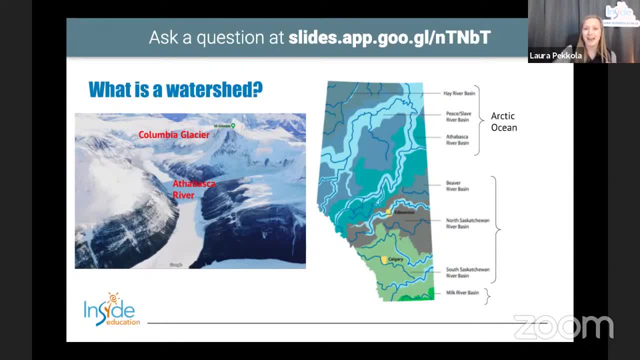 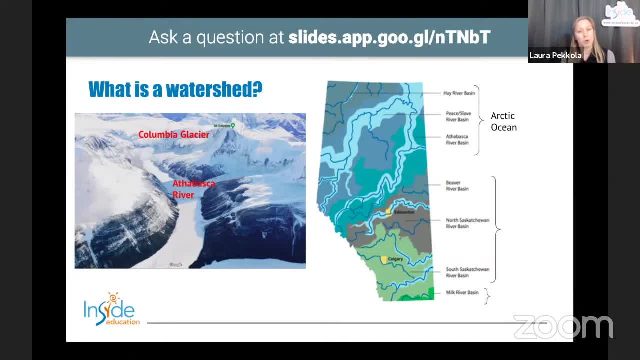 pollutants or medicines or hormones that end up in the water will get more diluted, But they are going to continue all the way down the river, all the way up to the Arctic Ocean, which which means that there's a lot of communities along the way that are going to be connected by whatever is. 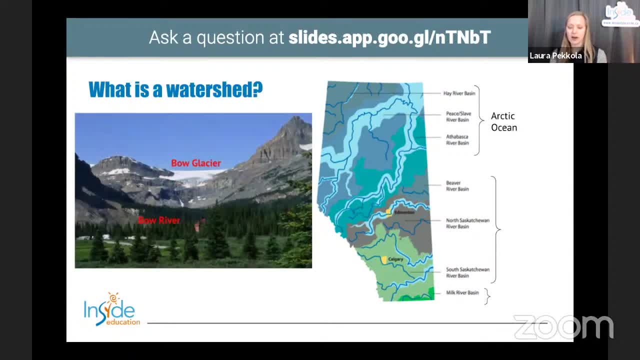 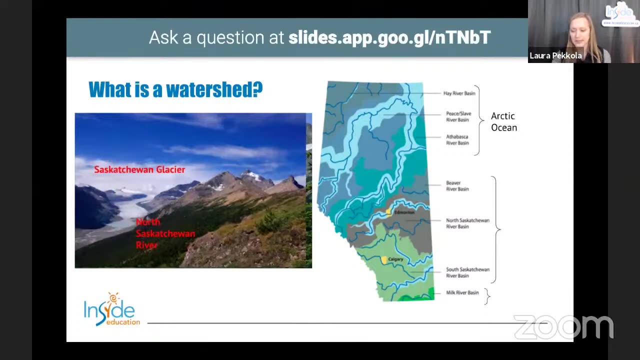 happening upstream of them. Now let's take a look here or down south, to the Bow Glacier and the Bow River. So the Bow Glacier feeds the Bow River and and the Saskatchewan Glacier feeds the North Saskatchewan River, which goes right through Edmonton. here And those head all the way. 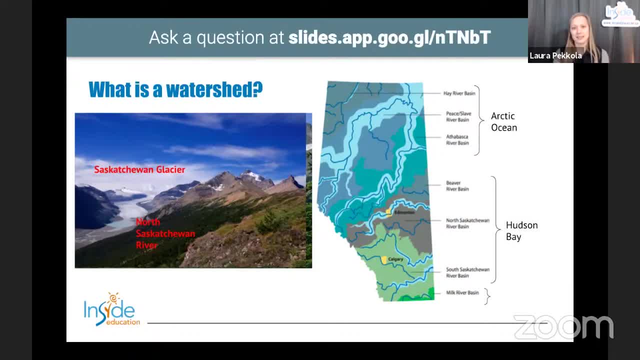 up to Hudson's Bay. So going back to that example of the medicines at the Gold Bar water treatment plant which is here in Edmonton, those medicines and hormones are going to end up affecting the communities all through Saskatchewan and Manitoba and then into the Hudson Bay area as well, And 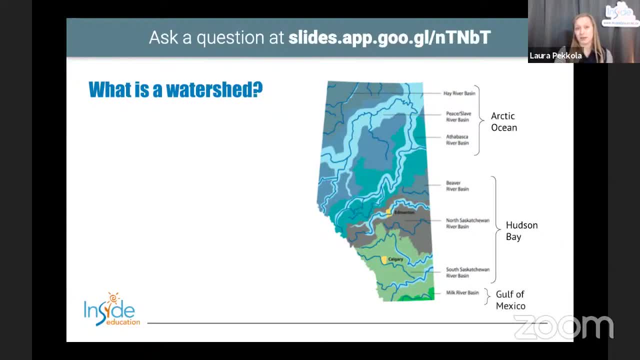 then, finally, we have our Milk River Basin at the bottom, which actually goes all the way down to the Gulf of Mexico. So, even though things get diluted when they end up in water, it is really important to remember that there are other communities downstream which will or may be affected by whatever we do. 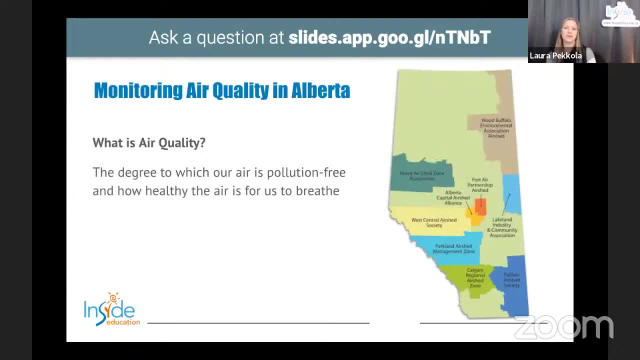 here And, similarly to watersheds, there's actually something called an airshed as well. So airsheds- you can see the airsheds of Alberta split up here- These are associations that monitor the air in these specific areas And then and they, so we don't actually have all of. 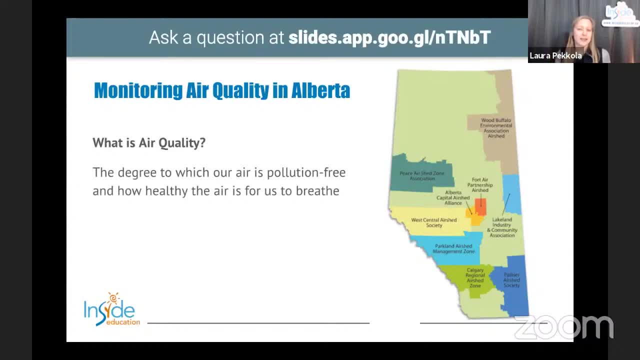 Alberta covered by airshed associations. Does that mean that these blank areas on the map are not part of an airshed at all? Of course not, Because I've noticed, at least, that there aren't too many walls between, say, or between Edmonton and Calgary that say, okay, you're entering a new airshed. 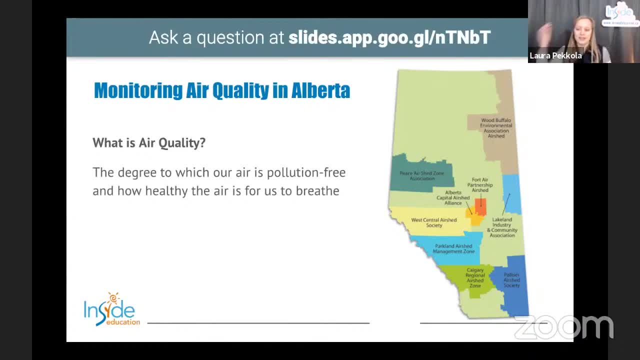 open up my plexiglass door and walk through. That's not how it works. This is just human created boundaries that allow for monitoring to take place, But air is going to move wherever it pleases because it moves quite easily. So an example of that is wildfires, which you've probably 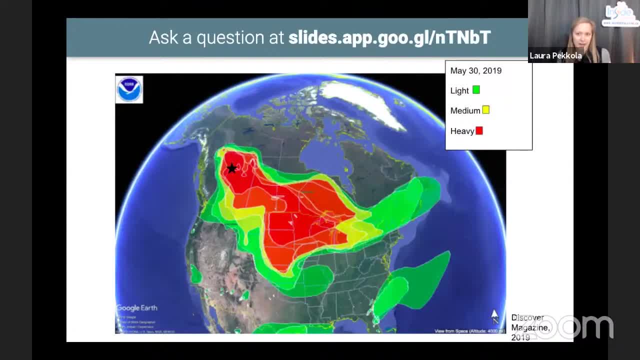 experienced at some point if you've spent summers in Alberta. So here is a map of, or an image showing the distribution of airsheds in Alberta. So here's a map of Alberta. So here's a map of of smoke from the high level fires in May of 2019.. So a year and a half ago. So that black star. 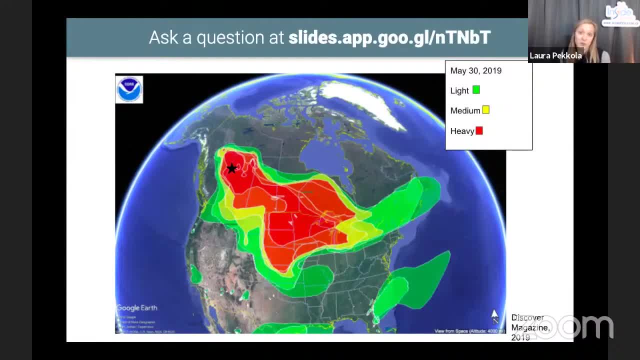 on the map is where high level is and where the fires were actually taking place. Now the red area is quite high concentrations of smoke, And then yellow is a little bit less and green is quite light. You'll notice that the smoke from that high level fire did travel all the way to. 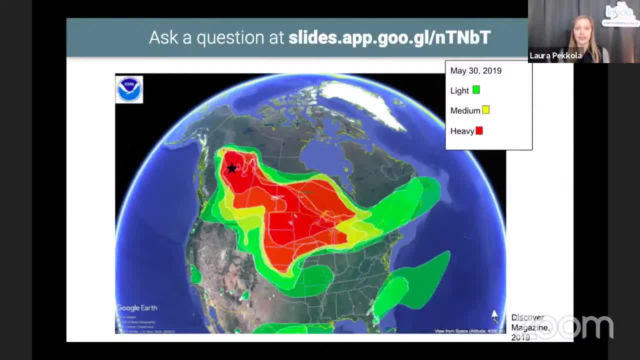 at a concentration or a thickness that was enough to even be noticed. So, regardless of the fact that that smoke moved from airshed to airshed, it still continued on west following the wind currents, and affected people east of us here in Alberta. So wildfires are actually one of the big ways that 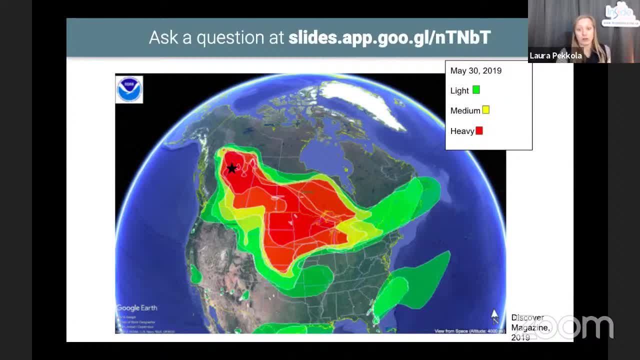 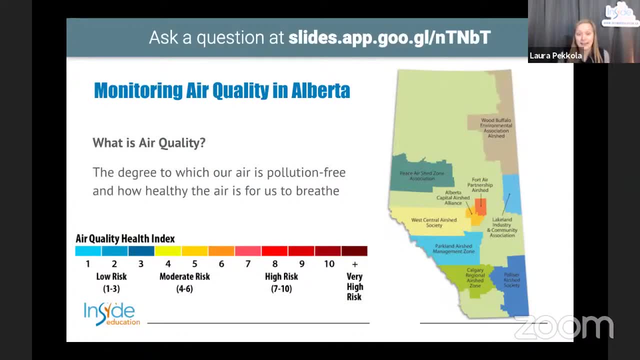 air quality can be affected, especially here in North America, And it's actually the main reason why our Air Quality Health Index might increase or show poorer air quality when, especially in the summer. So air quality is the degree to which our air is pollution free and how healthy the air 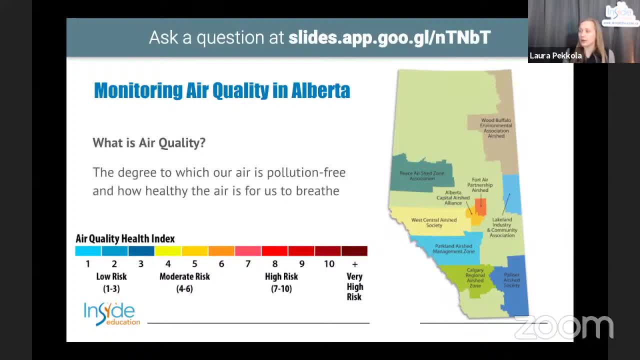 is for us to breathe. So if you look outside right now, if you had to guess, what do you think that air quality is today? Is it pretty good or is it quite poor? To help with actually quantifying this, these indexes, called the Air Quality Health Index, have been developed so that there's actually a 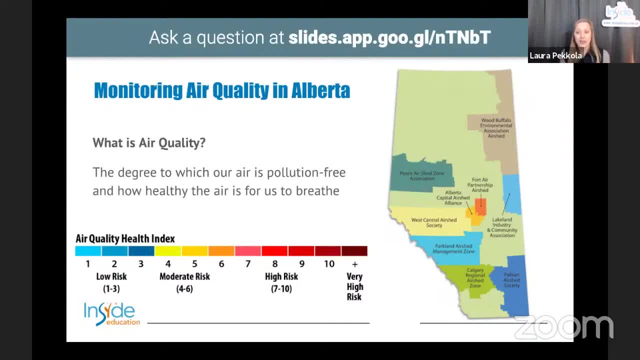 number scale. So the AQHI is calculated based on measurements of various pollutants. In for the national AQHI it measures ozone, particulate matter and nitrous oxides and then does a calculation to figure out how big of a risk to human health it is. And then in Alberta, 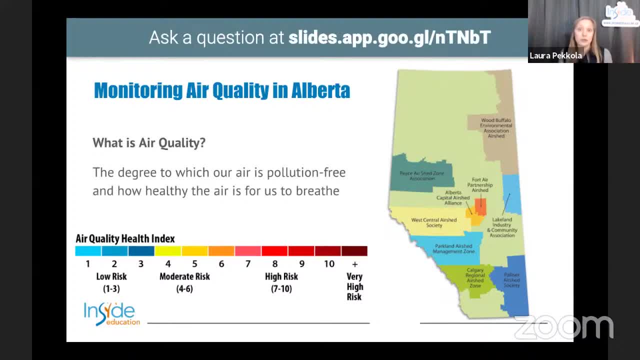 we've added a couple of other pollutants that are kind of locally relevant. So depending on where you're looking at AQHI, it might be measured in a slightly different way, but it does give us an idea of how healthy the air is or how risky the air is, I suppose. 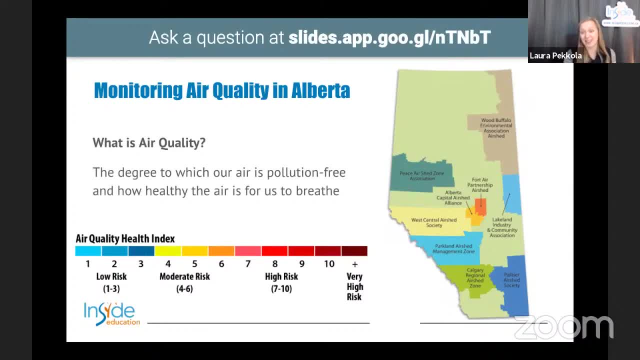 So I see that someone responded that they bet the air quality today is very good. And here in Edmonton I'm looking out, I don't see smog. I don't see smoke in the air. So I would agree It seems pretty, pretty good. So that means that it's pretty low risk, or I'm guessing that's pretty low. 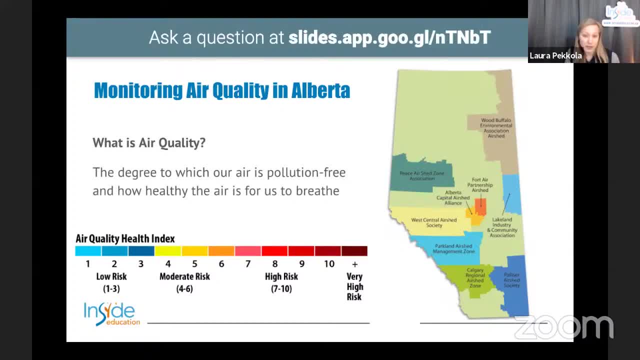 risk to be outside. Now I actually checked the AQHI website and that is the case. The AQHI here in Edmonton is between the three And a four based on the calculations at the different monitoring stations in the area. So that means that it's very low, maybe getting into moderate risk, but but pretty good to be outside. 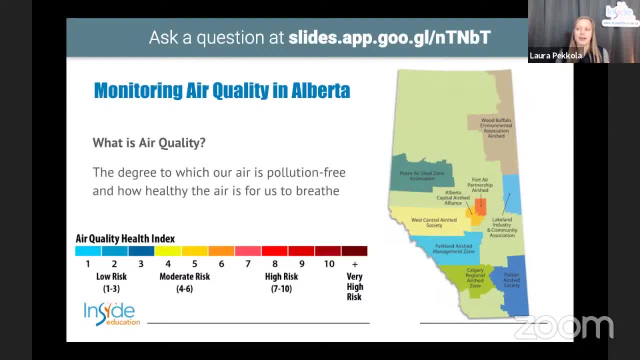 So maybe you've remembered some days when you've had to have an indoor recess, even though it's nice and sunny outside. it's warm out and you can't figure out why. Well, when AQHI gets above seven, it can cause a high enough risk to 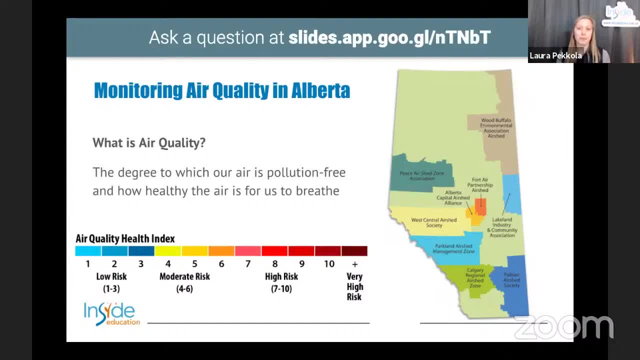 It can cause a high enough risk for students or- and also adults, anyone in the public- that it's better to stay inside and not exert yourself too much with too much activity. So we can actually check the AQHI in our weather forecasts and it can help us decide whether to spend a lot of time. 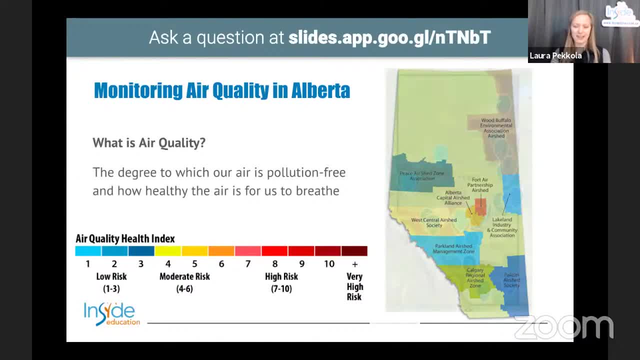 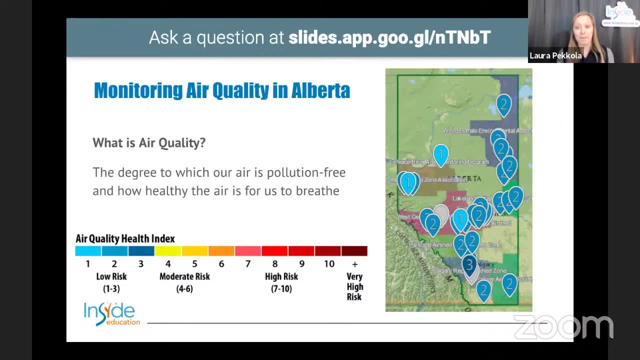 outside or kind of hunker down inside instead. So here is a picture of the map that you would see If you went to the AQHI Alberta map, so it will show all the monitoring stations across the province and then you can see real time data from there, as well as predictions for the following day as well. 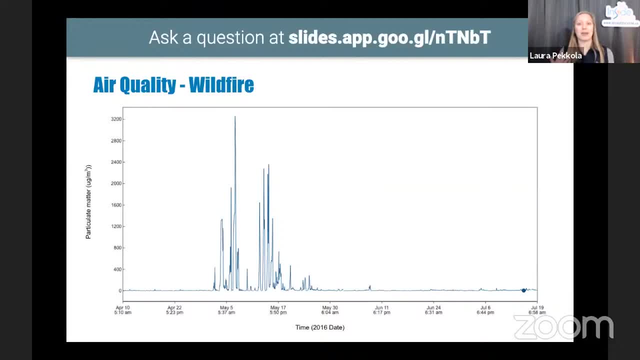 So an example of how air quality can, or how AQHI can be measured and where we've seen big spikes in AQHI, I'm going to take us back to May 2016, when the large wildfire took place in Fort McMurray. So this graph is actually showing particulate matter, Remember, which are those tiny airborne particles that can get into our lungs, and at the beginning of May, here you can see that the amount of particulate matter in the 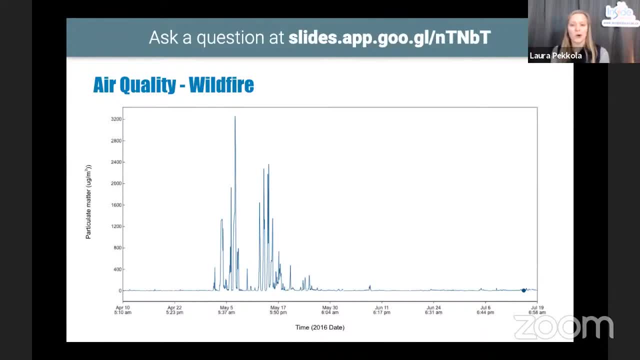 In the air really spiked. Okay, so that is because there was a lot of combustion, a lot of burning going on, a lot of soot being released, and it caused the particulate matter to spike And then it stayed there. So, and it stayed high for a lot of that summer, especially at the beginning when the fire was quite strong. 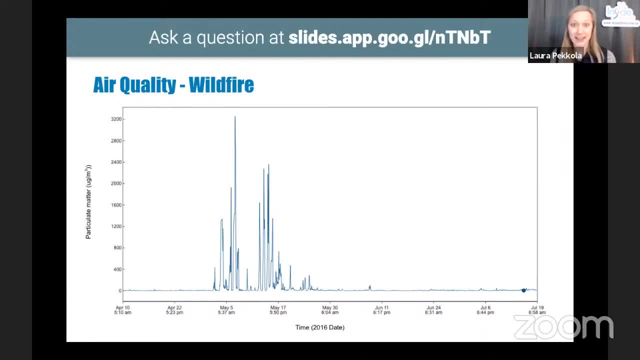 So at this point, when the particulate matter spiked like this, the AQHI actually went over 300. remember on that last slide we saw the scale usually goes from 1-10 and anything over 10 is quite quiet high risk. 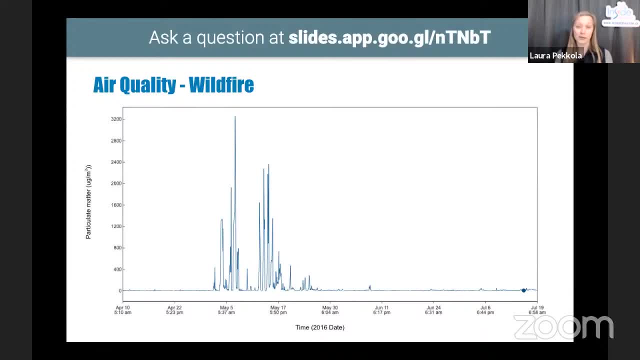 Well in Fort McMurray at the time of this wildfire we were over 300, because there was so many particulate matter removed during the year that it got all over water. So here could see publications onіль and a lot of evidence that we had from these wild fireworks. 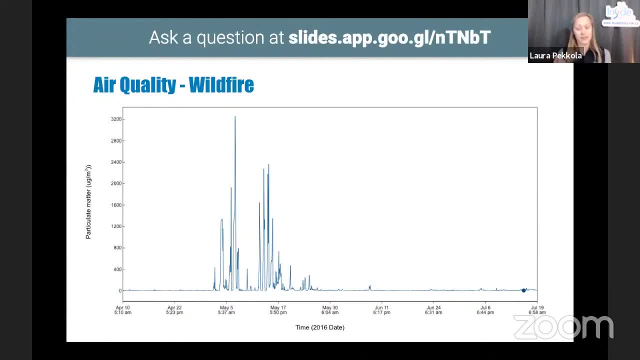 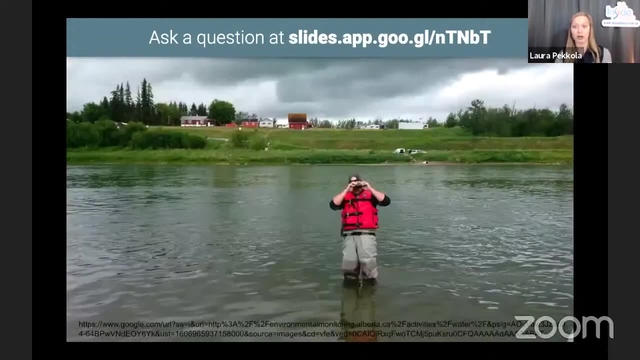 wildfire, wildfires, water- much particulate matters, especially in the air. So, yeah, really helpful to have that tool to be able to measure the risk of the air around us to make sure that we can keep ourselves healthy. Now we can also look at water quality monitoring. It's done by Environment and Parks here in Alberta. 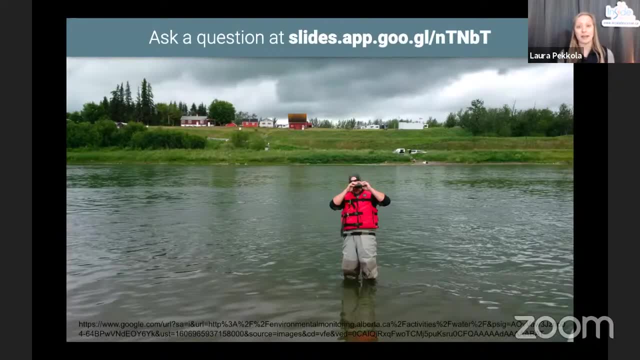 as well as a variety of partners, partner groups that exist in our province. So they monitor the water to ensure safe drinking water. They monitor for pathogens in the water that might make you sick or itchy if you swim or enter the water Again in that water. presentation from a couple. 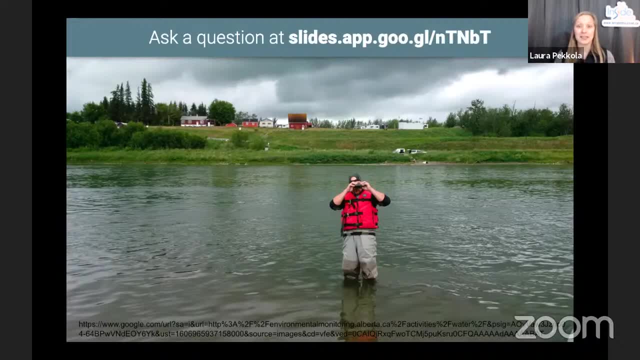 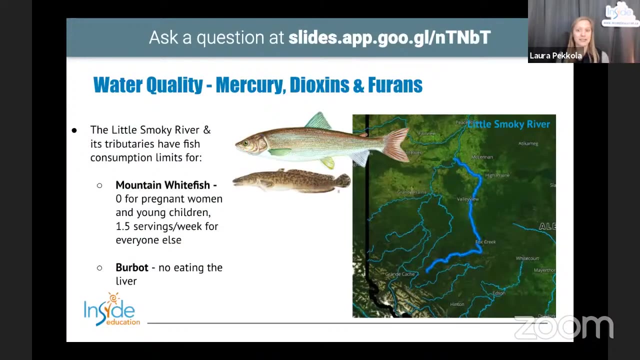 weeks ago, I believe Andre talked a little bit about swimmer's itch, So if you're interested in that, go check that out. And also they monitor the water for the health of the environment as well. So an example of why water quality might be important is 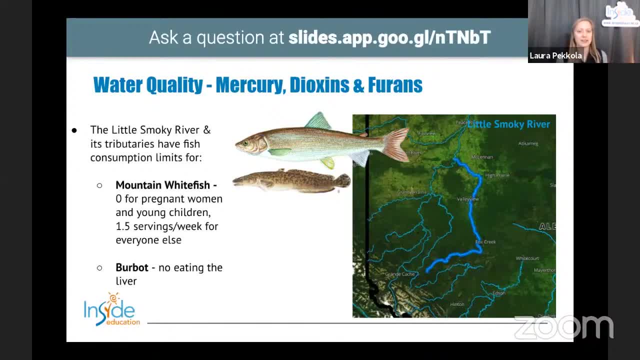 looking at fish in the Little Smoky River and its tributaries. So they actually have some consumption limits of these fish. So the mountain whitefish and the burbot, because of- well, for some reason, Why do you think they might have consumption limits on some of these? 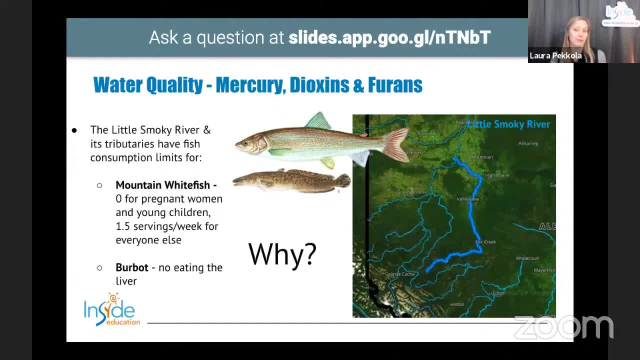 different types of fish. I'll let you think about that for a moment. So if you are an avid fisher, this is one of the things that you can take a look at before you go out fishing: to make sure that there aren't consumption limits in the area that you're. 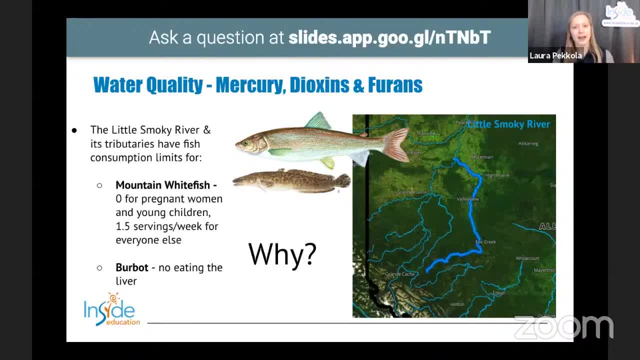 fishing in, And really the main reason for that is to keep you healthy. So these fish in this area have been found to have high amounts of mercury in their livers and in their fatty tissue, And the reason why mercury can be a problem is kind of like we were talking about the microplastics. 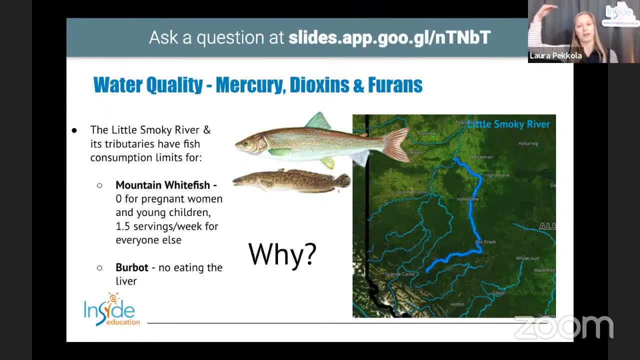 and the invertebrates is that because these fish are kind of higher up on the food chain, they eat other organisms that have mercury in them and then it accumulates within their tissues, in the fish tissues, And that process is called bioaccumulation. So the higher up an animal is, 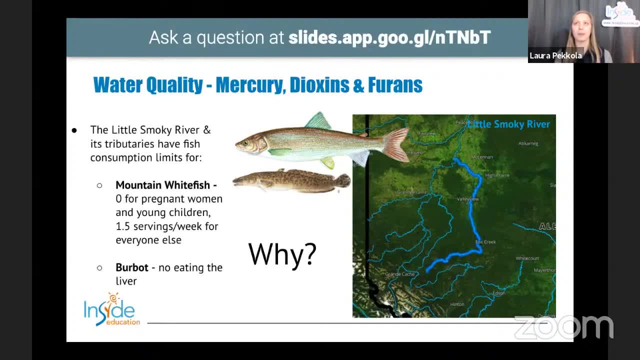 on the food chain, the more of these chemicals it might end up with in its body as well, And I see that microplastics and harmful chemicals were some of the ideas that you had. so, absolutely perfect. That is exactly what we are considering here And again this case. 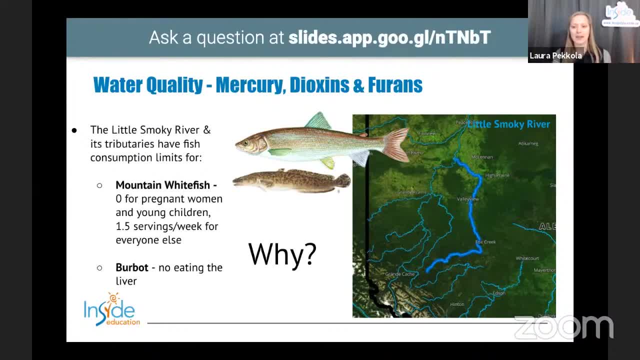 specifically mercury and mainly it's coming from human sources such as burning coal and also burning waste. that might release methylmercury And this ends up in water bodies through runoff, for example, And it's really easily absorbed by the fish. So the mercury in the air isn't a problem. 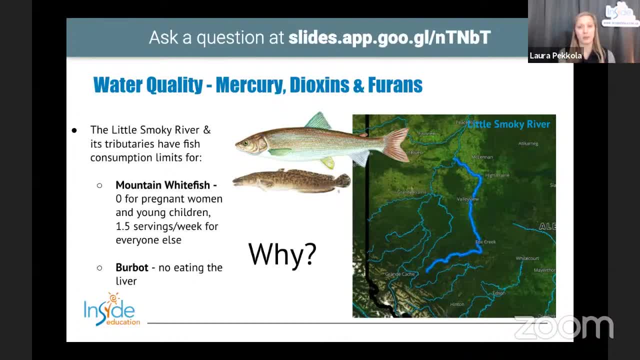 it's more of a problem once it's converted into the methylmercury, which ends up in the water system as well. And then the dioxins and furins which you can see at the top of the screen there as well. they are toxic, airborne substances from burning organics and wastewater discharges from. 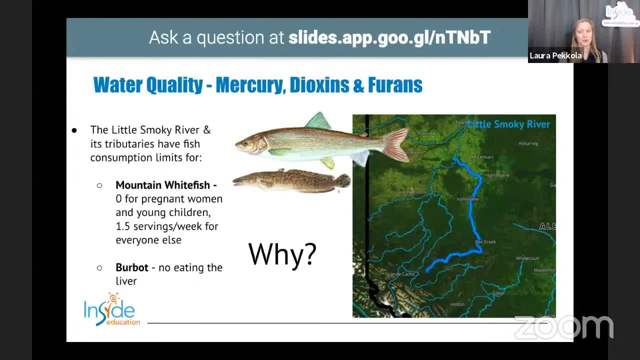 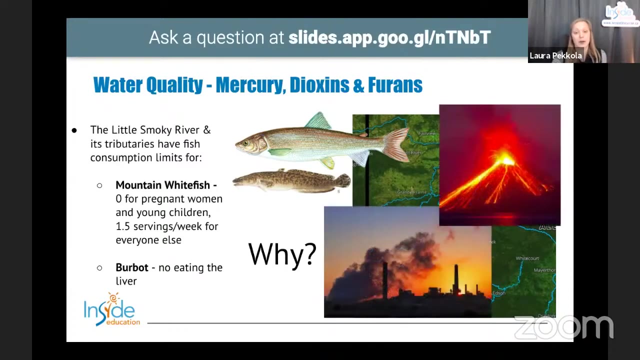 industrial sites. So the largest source of those is burning of municipal and medical waste. so in Canada Also from producing iron and steel and burning other fuels as well. So they also work their way up the food chain and can be stored in the body. So something to keep in mind as we take things from the environment, because they can have. 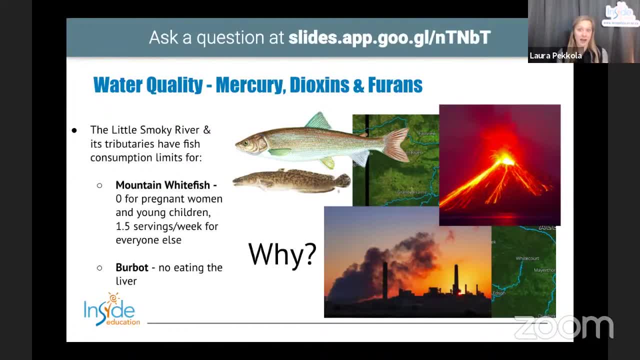 toxins within them, And they can also come from natural sources. So volcanoes can emit some of these these toxins as well. So just because something is a chemical doesn't mean that it can't come from a natural source. The main issue with some of these chemicals and pollutants is that humans 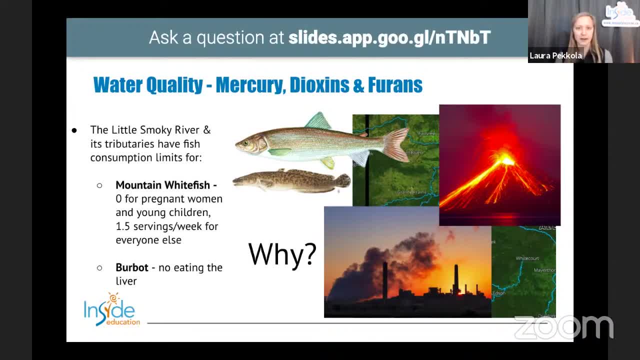 are adding even more to the environment than would naturally be there, And then that can be the main challenge And that's also the part that we can do something about. So that's what we really want to focus on. My final example: I want to look at emissions in our oil sands region specifically. 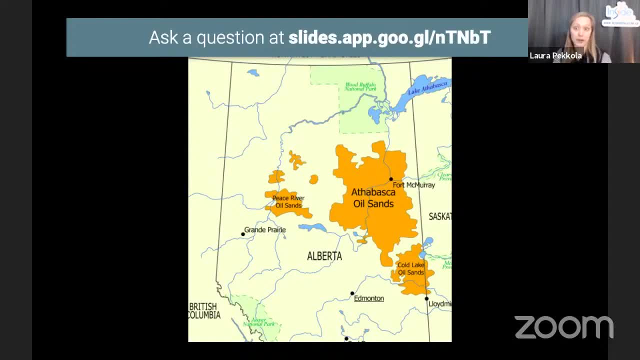 the Athabasca oil sands, Which is in and around Fort McMurray. It's our biggest oil sands area, has the highest amount of surface mining And there's a lot of production of oil or a lot of refining and upgrading of the oil that happens there, Which means that sulfur can actually be emitted through these. 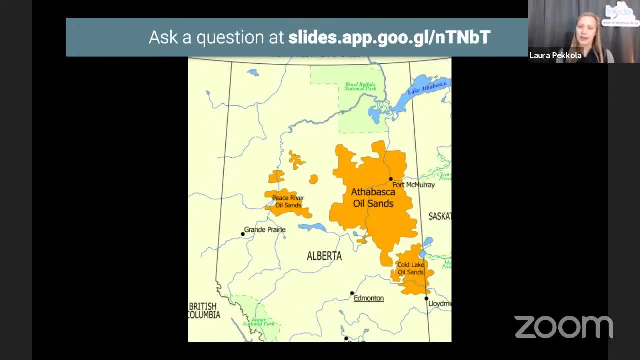 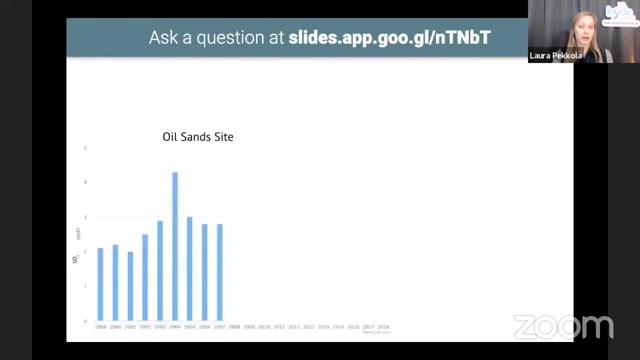 processes. So, thinking back to that map that we looked at at the very beginning of the presentation, the main source of sulfur is industrial process, Especially in fossil fuels, which are naturally high in sulfur. So let's look at this graph- and I'm going to show you a series of graphs- to kind of see what might be happening up in that area. 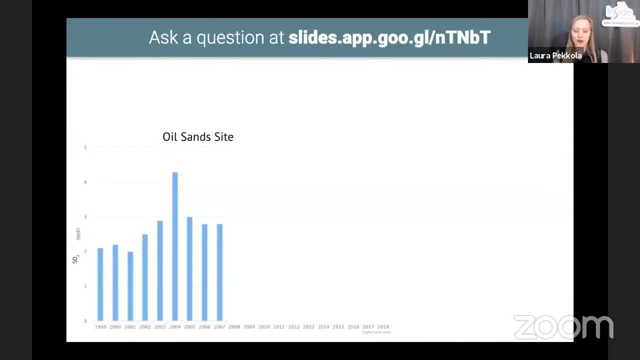 So this first graph shows how sulfur emissions at an oil sands site have changed year to year. So for the most part- other than this higher blip in 2004,- they've remained pretty level correct. So we can also look at how much oil has been produced by the oil sands area. 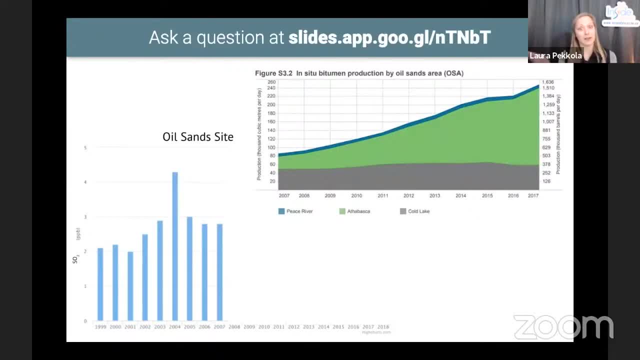 So that big green wedge is the Athabasca oil sands, which is the Fort McMurray area, Which is where these sulfur measurements were taken as well. So this graph starts at 2007,, the top one showing the oil sands production. What do you think happens to sulfur emissions? 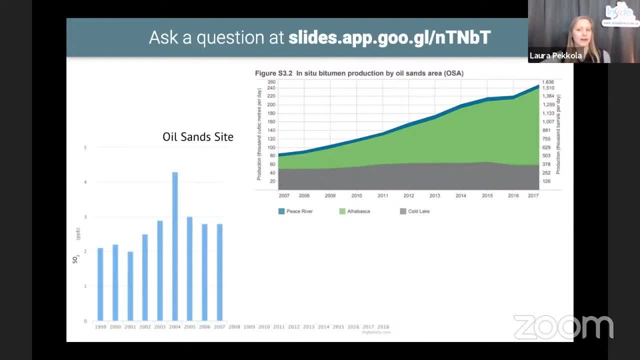 if our oil sands production is increasing. I'll give you a moment to think about that. So we don't know what the oil sands production looked like before 2007, because this graph starts at 2007.. But based on what you know about where sulfur comes from, 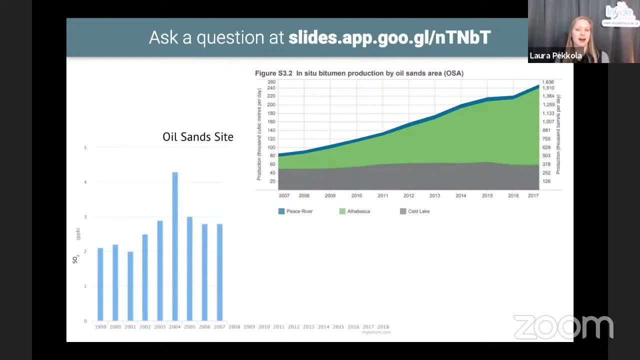 what do you think might be the story from 2008 onward when we look at our sulfur emissions? Let's see if there's any brave people out there. So if you're a little confused and unsure, that's totally okay. My guess would be that the sulfur 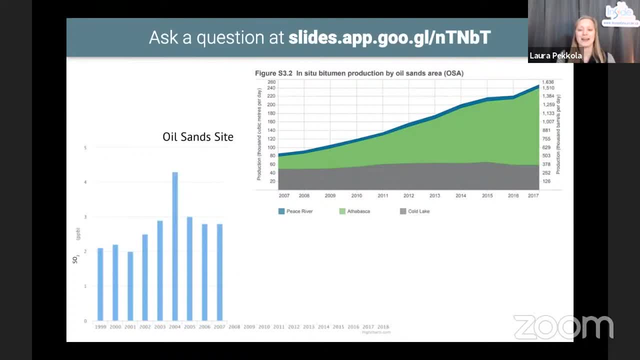 emissions would start increasing, And because the oil sands production is increasing as well. But let's take a look at the story. Turns out that the sulfur emissions actually stay pretty steady even though the oil sands production is increasing. Now why would that be? I would have expected the emissions get higher. 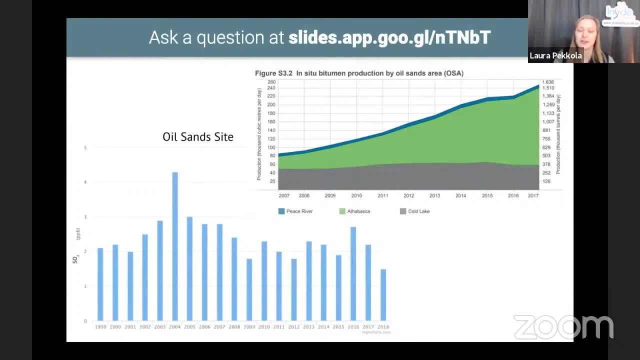 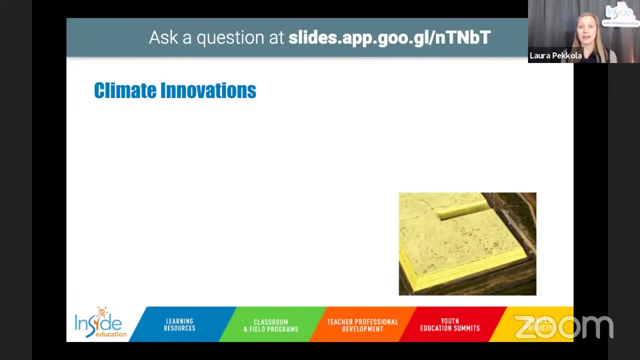 but just because our production is increasing doesn't mean that there's not technology and innovations that are also happening to try and reduce our negative impacts on oil sands. So we can't really be sure that we're actually reducing the impacts on the environment. So one of the things that is taking place especially in oil sands production, 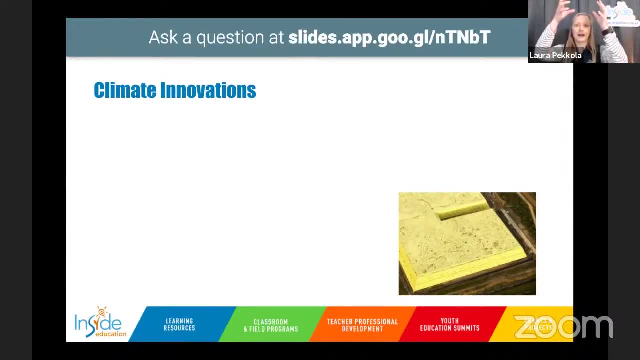 is sulfur scrubbers. So by putting these scrubbers into the chimneys that come off of these plants, they can actually take the sulfur out of the emissions. that would end up in the air and create solid blocks of sulfur out of it. So on the screen is actually one of these solid blocks of sulfur. 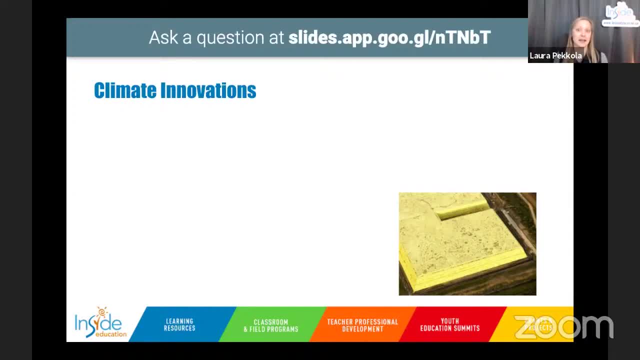 that are piled up in and around the oil sands plants. So they've taken it out of the air and are storing it as a solid. Still a bit of a problem. We need to figure out what to do with that solid, but at least it's not polluting the air. 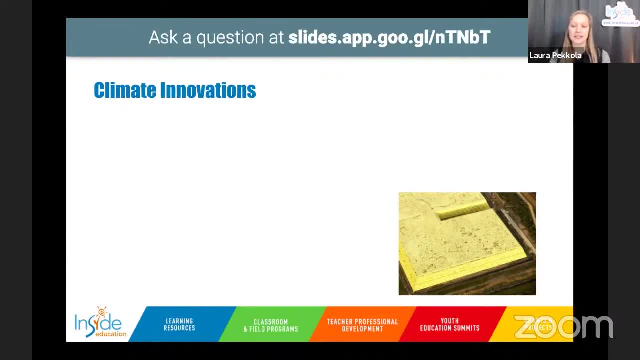 Some of the other innovations that are helping our air quality specifically have to do with carbon capture. So we don't talk much about carbon, but when we burn fossil fuels we do release carbon dioxide, which is a very, very potent greenhouse gas. 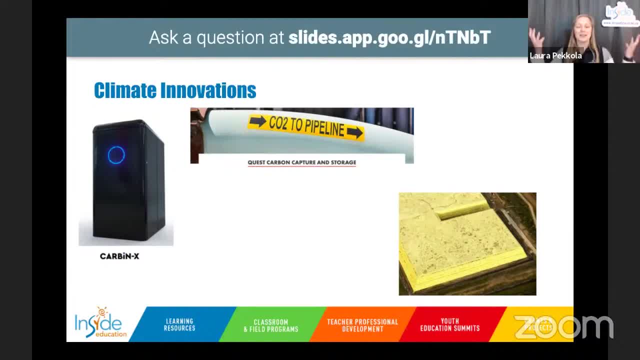 So there are some technologies out there that are being developed to actually take that carbon out of the air and make something useful out of it. So the CarbonX on the left side of your screen. there they actually take the carbon out of the air and then they produce a potash out of it. 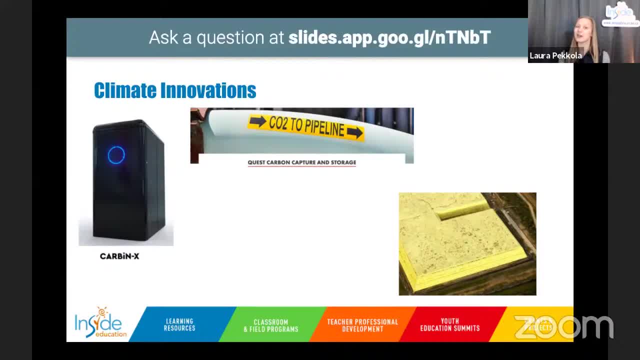 and they can actually make soap out of that potash that they are taking out of the air. So this is an Alberta-based company, so maybe if you're looking for some climate-friendly, local Christmas gifts, you can look into some CarbonX soaps. 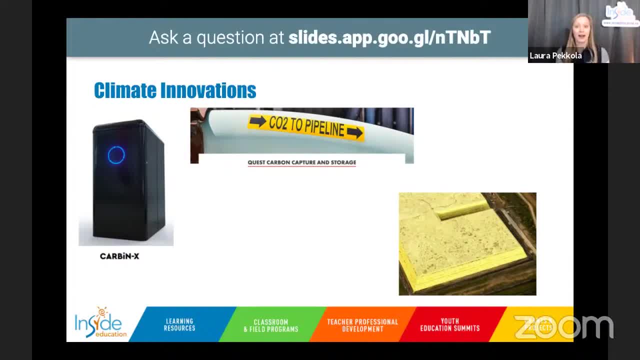 The CO2 pipeline is from the Shell Quest carbon capture and storage facility, So it's in Fort Saskatchewan, just outside Edmonton here, and they are taking carbon out of the air from the or out of the emissions from the Shell bitumen upgrader. 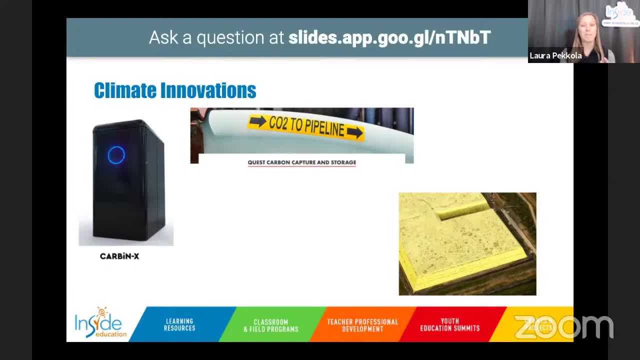 But they are taking out an equivalent of a million cars worth of carbon out of the air yearly, So doing a pretty good job of reducing carbon emissions there. There's also electric buses, As here in Edmonton, 40 were purchased and a few of them went on the road in August of 2020,. 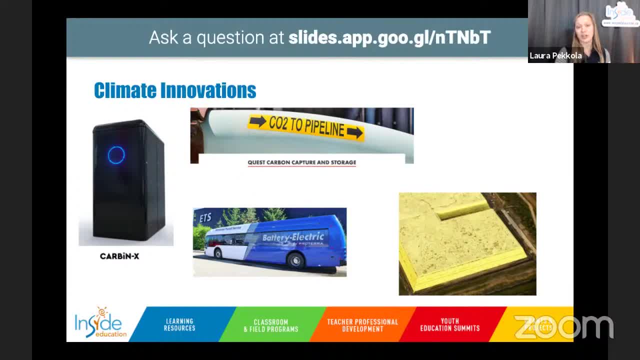 which is pretty cool. So that's reducing our fossil fuel-generated or fossil fuel-burning-generated generated carbon emissions as well, And then something that we can do in our own homes is looking for these energy efficient options which reduce the amount of electricity that is needed. 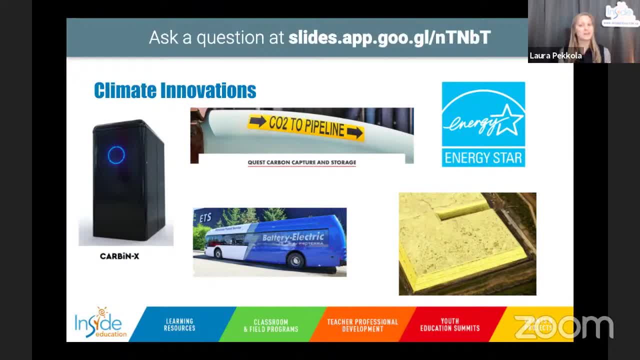 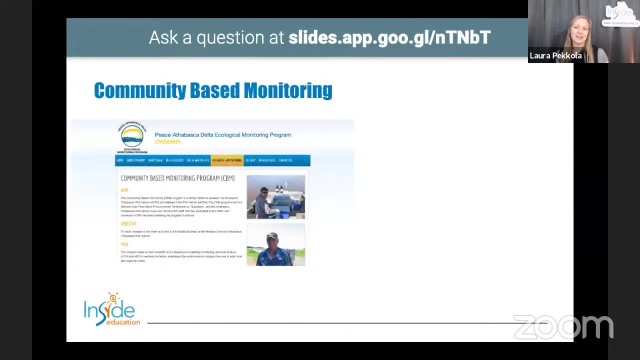 because where does Alberta's electricity come from? Mainly from burning natural gas, which again does produce a lot of carbon. So lots of innovations in the works as well. Now, one last thing I want to talk about before I wrap up for the day is about community-based. 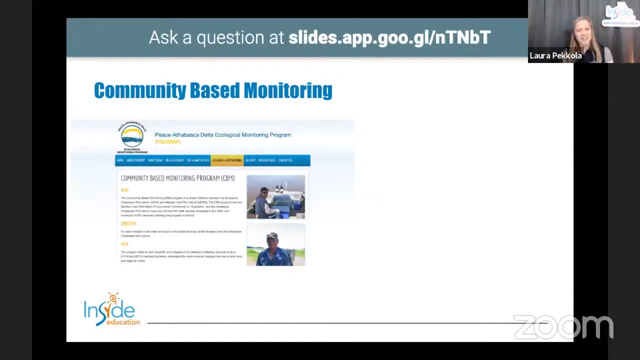 monitoring. So far, we've talked a lot about the science of monitoring and ways of measuring in the environment, and I'm wondering: does that tell the whole story? Well, Indigenous knowledge can actually fill many gaps about these areas that are being monitored, as the history of that. 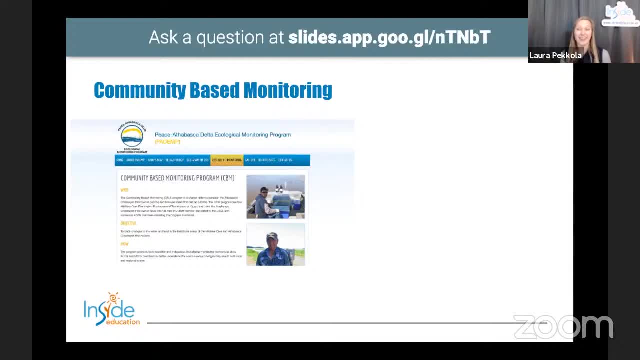 knowledge and of the people of that area reaches back thousands, Thousands of years. So the way of seeing and learning about the world in Indigenous cultures is different from the way that I'm assuming many of us are most familiar with, which is the scientific method. So different information can be gathered by seeing the world around us in these 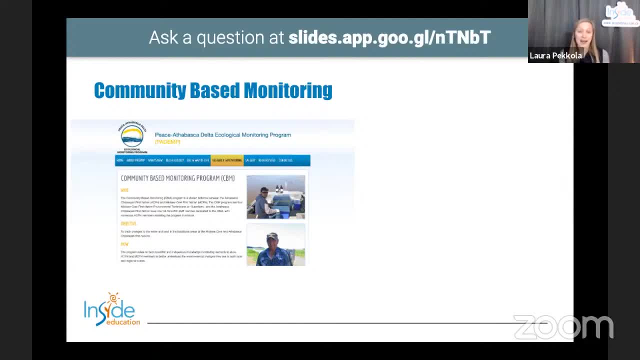 different ways. Community-based monitoring does just that, Tries to incorporate the Indigenous, traditional knowledge of an area as well as the scientific measurements and measurements of the area. So the way that we can see the world around us in these different ways and process that we can, we can put into use and then it kind of gives a more complete and total 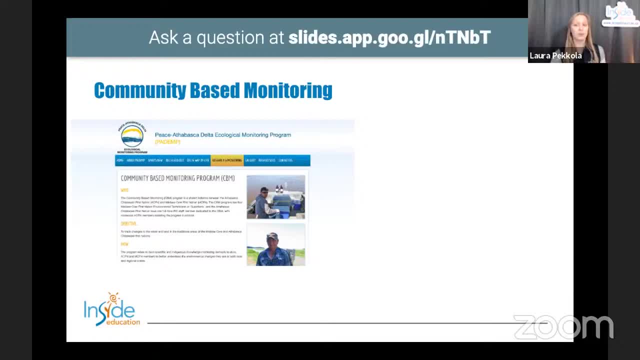 story, which I think is really awesome. Community-based monitoring also allows the communities themselves to direct the reasoning and the the way in which the research is done, which can be incredibly important in ensuring that they are getting the information that they themselves want about their own traditional land. 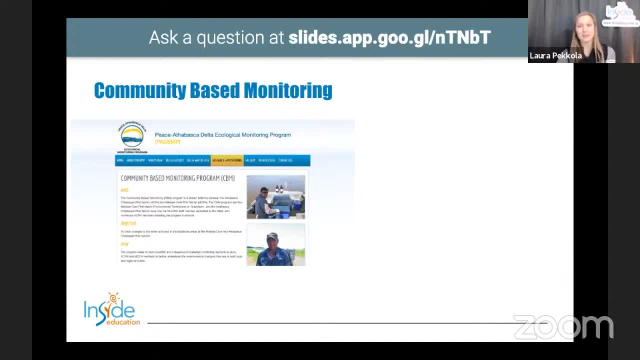 ens and communities as well. So there's, when you at the tip, a few examples of this happening in Alberta. So the first one is up on the screen there. It is the Peace Athabasca Delta environmental modern monitoring project, or uh padimp, as you see, And it is a um, it's a bunch of the different Indigenous. 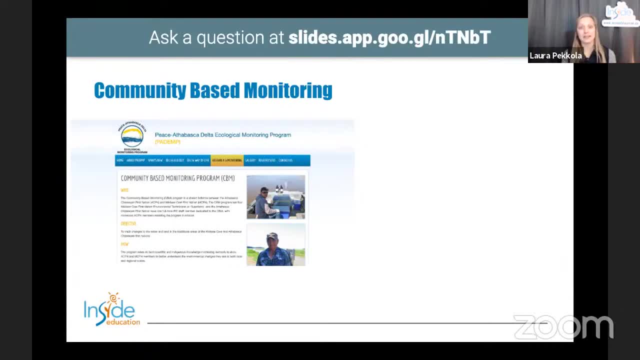 groups from that area or in Bulllets later on. Orange, dur, silver, deeper water layer um scientists and monitors to uh gather information about the water and traditional lands of their area. Also, Wood Buffalo Environmental Association is working with indigenous communities around Fort McKay to look at the impact of air quality on the berries that are found on their 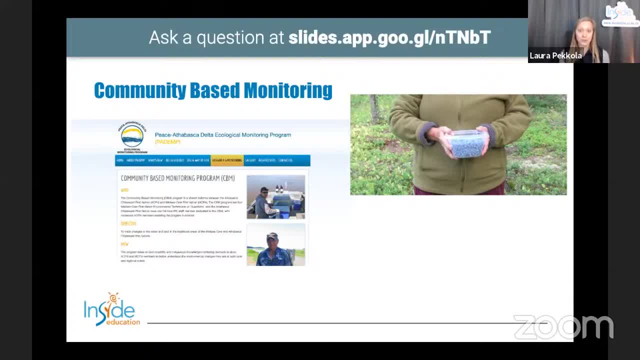 traditional lands. So those berries are an important uh food source for uh the indigenous peoples of that area and have traditionally been a food source. but now, with the oil sands operations in the area, they want to look at if any of that, um, any of the pollutants that might be in the air. 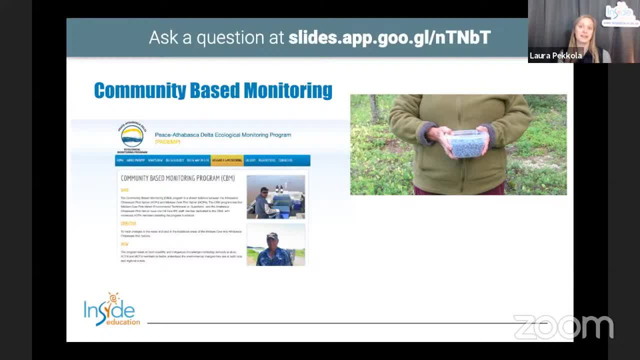 if it's going to affect the health of the berries and then also if that could transfer to the health of humans as well. And finally, uh, there is fish monitoring taking place, uh, in the Cold Lake area with the Cold Lake First Nations, um, so that they could know more about the populations of fish in. 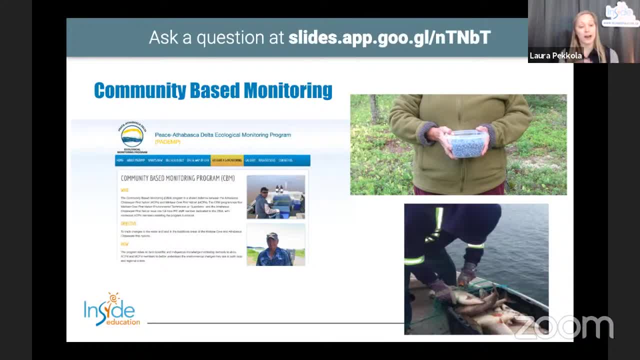 that area. Something really interesting for any of you who might be- uh might be interested in um getting into monitoring. uh, there's actually a community-based monitoring program at Keanu for indigenous students to learn the scientific methods as well as the indigenous land land-based perspectives. 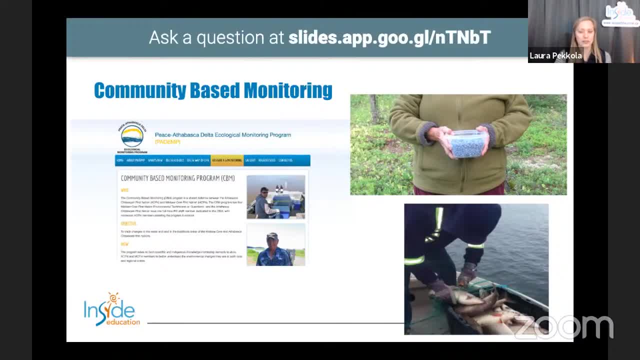 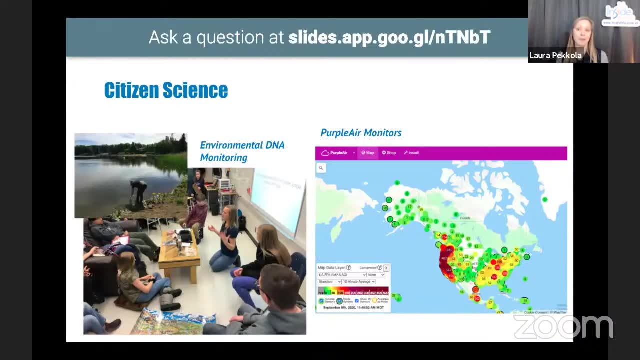 on monitoring as well. So something pretty cool to look into Now: ways that you can get involved right now. uh, citizen science, it's an opportunity for uh, the public And students to get involved at a community level. So I'm going to give you a couple of examples here. 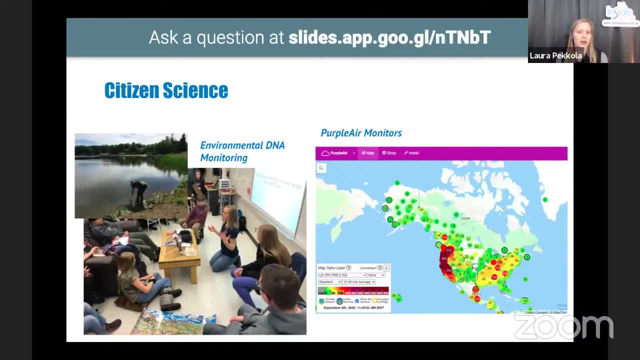 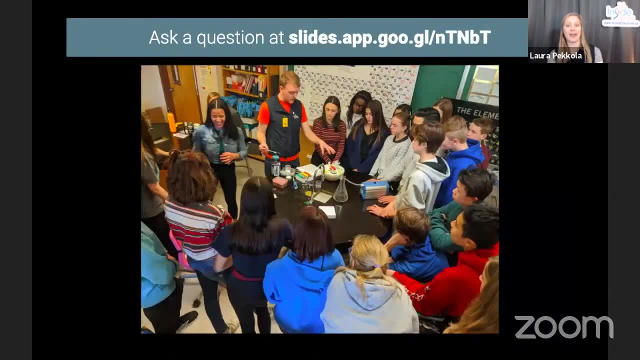 Uh, the first one is the environmental DNA monitoring in water, which, again, Andre talked about in that water presentation. So I uh suggest you take a look back at that if you're interested in more information. But uh, here's Colin, uh at St Matthew's School in Calgary and, uh, we once in 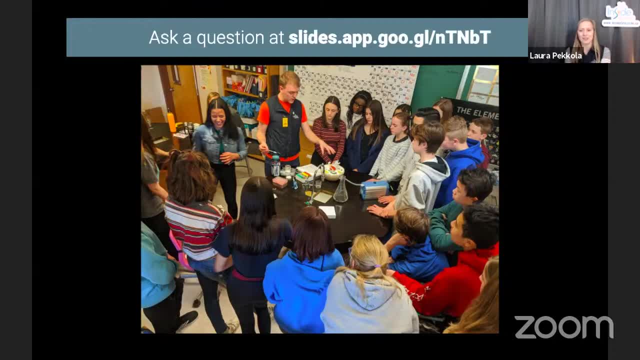 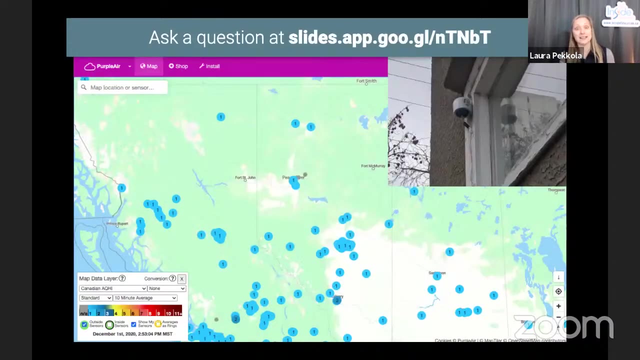 person visits uh start up again. we'll be able to bring these machines into the classroom and show students the process of actually extracting that DNA uh from uh from water samples, and then explain how that can be used for monitoring as well. And then Purple Air- uh is an air monitoring. 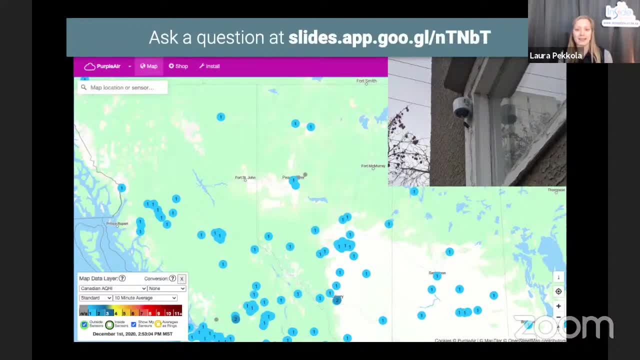 program that is taking place at the community level. Uh, these are different sensors from the Alberta sensors which I mentioned with the AQHI, But these sensors, um, you can possibly get one onto your school or onto your community league. I know, in um, in Edmonton, uh, community leagues are being offered these sensors for free. So I'm actually 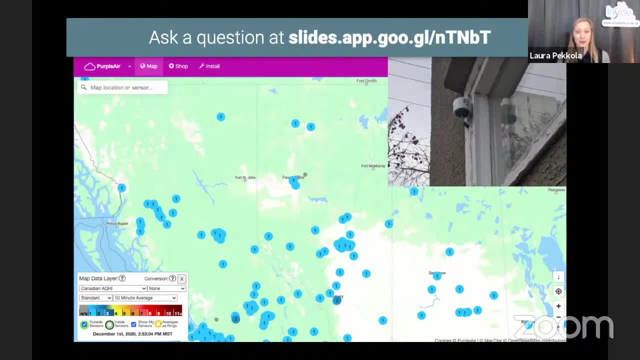 going to meet with my community league this afternoon to get one put onto our building, which I'm really excited about, And in the photo there on top of the mac you can see the one that is installed at the inside education- inside education office right here. So kind of just gives some more. 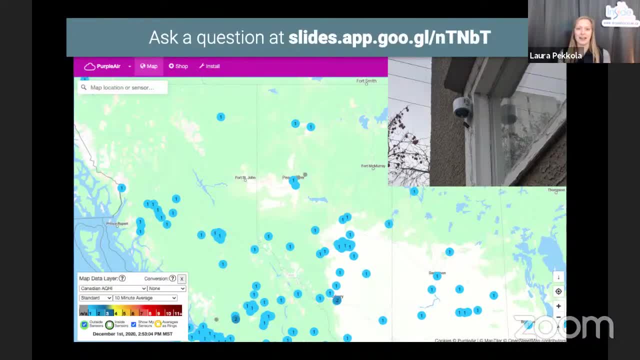 regional data about air quality And uh, and you can look at any place across the world um for what the air quality model is. It might be there as well, So definitely check it out if you're interested. Purple Air is what you have to google and then you can take a look at air quality anywhere across um across the world. 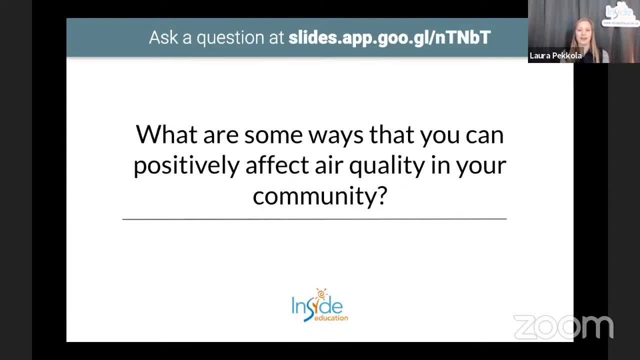 So, uh, what are some ways that you can positively affect air quality in your community? Um, just put in a couple thoughts into the Q&A because I would love to see what you think. But, uh, as I'm waiting for that to be populated, I'll share some of the thoughts that we gathered. a. 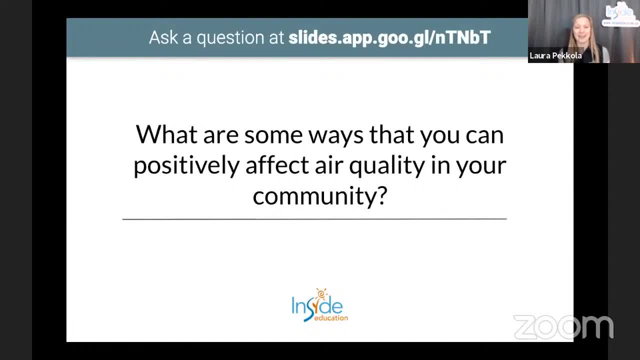 couple weeks of weeks ago. So I'm going to start off by sharing a little bit about, uh, how we can take care of our water quality. So, uh, we can make sure that our water is healthy by reducing the amount of water we use, by, maybe. 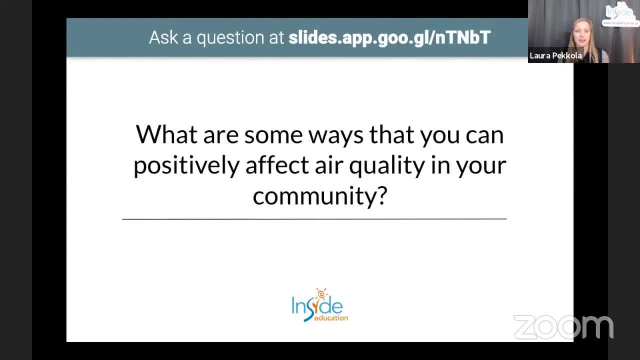 taking shorter showers and using a rain barrel to collect rain water to water our gardens instead of using hose. Uh, we can walk more and drive less, so that we're putting less pollutants out into the roads as well, And we can reduce the use of pesticides on gardens and just do some weeding. 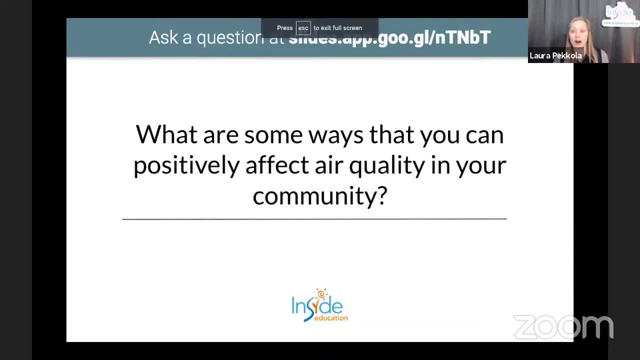 that way, those pesticides don't end up running off into our uh, into our environment. So let's see, oh awesome. someone says to take care of our air quality so you could bike or walk to school. So that is an awesome idea. and a couple of uh, my colleagues. 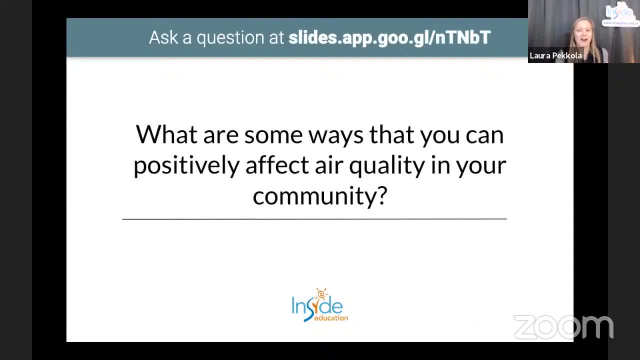 also mentioned that that would be a great way to take care of our- uh, take care of our- air. So Julie and Andre both had that to say. Um, Steve also says that you can just get a test list, so add that to your Christmas list. Uh, maybe not possible for everyone to be able to get one of. 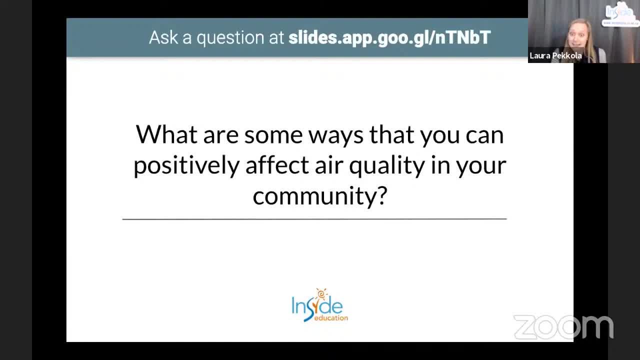 those, Um, use less electricity- awesome. so then that means that we're putting, uh, that there's less pollution being put out into the atmosphere because, uh, we're burning less natural gas. What else we could maybe put idle free signs, uh, around your school to make sure that cars. 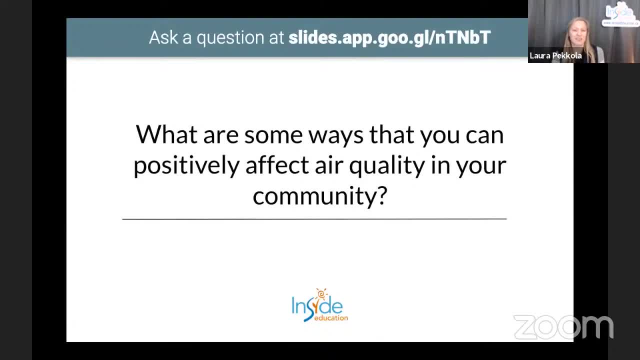 aren't idling or running without moving. uh, because that's a uh a way that pollution is put into the air, as well Any others. My favorite thing is you could take something that you heard here today and you can tell someone something interesting about air quality here in Alberta, because the more we can get others to care about 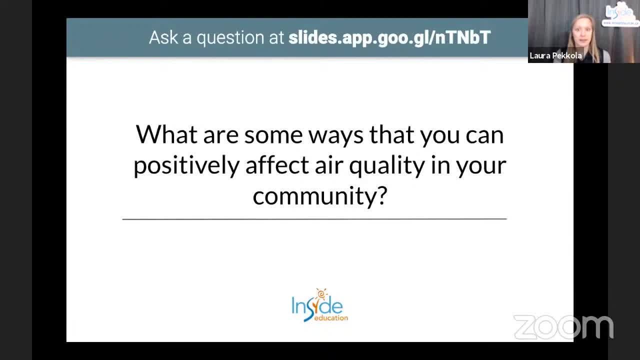 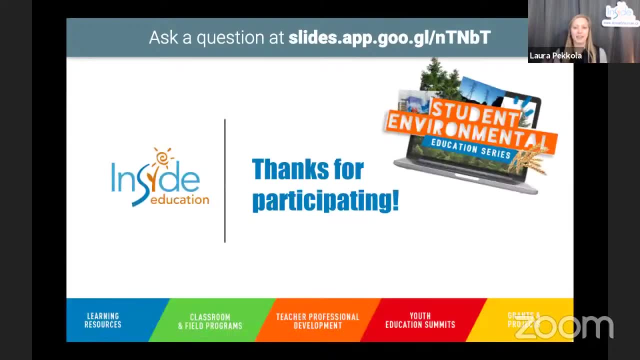 the topic, the more likely others are going to do something to take care of it as well. So that is just about, uh, all the time we have. So I want to thank you for participating in our final Student Environmental Education Series um webinar of the fall. um, stay tuned to. 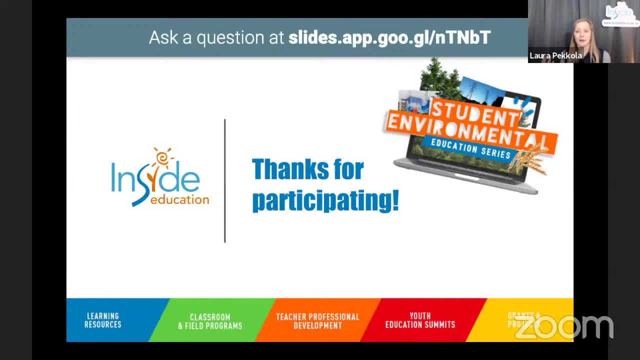 our YouTube page if you have other um, if you do have, uh, or if you want to see other presentations as well. There's lots of videos on there and, uh, there might be more coming, uh, in the new year, And before I sign off, I'll just double check to see if there are any questions. Oh, awesome, I see that there is one asking. 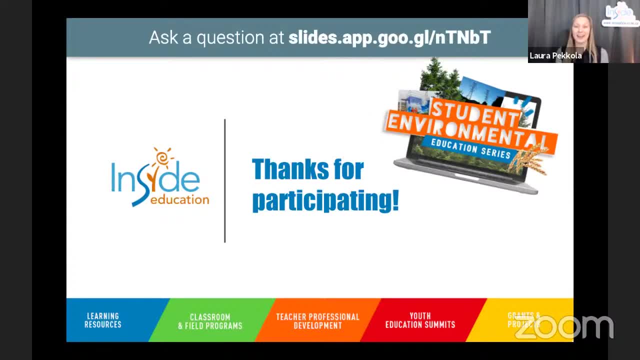 how can we help with the microplastic problem? That is a really good question and a really tricky one as well, because plastics are all they're in our life. We use them all the time. So one of the ways that we could maybe help with the microplastic problem is reduce the amount of. 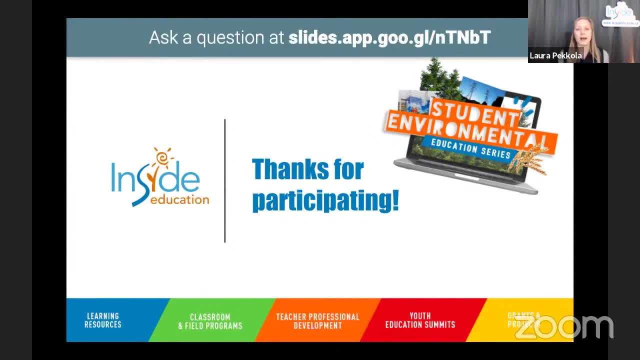 plastics that we use, So in some ways, like our car tires, are going to have plastics in them. There's not a whole lot we can do about it, but maybe we can choose what types of clothing we buy. try and buy natural fibers instead, Or maybe even with grocery bags if you have your own.